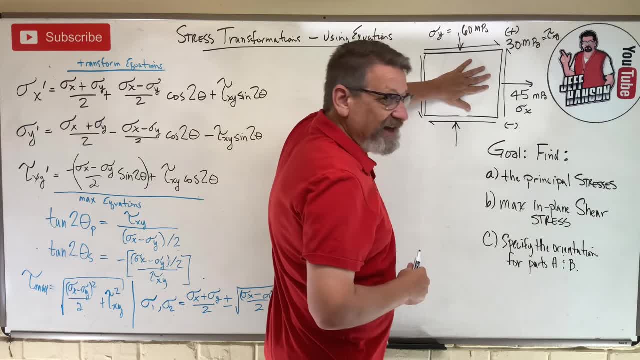 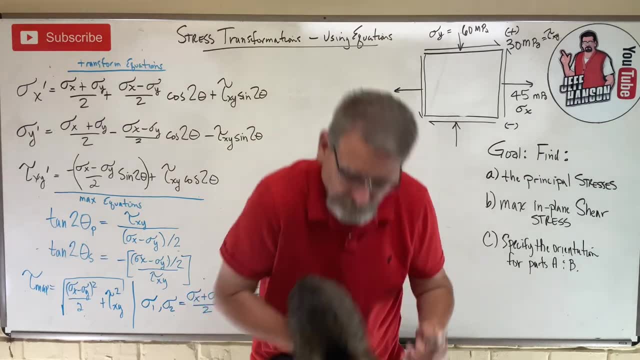 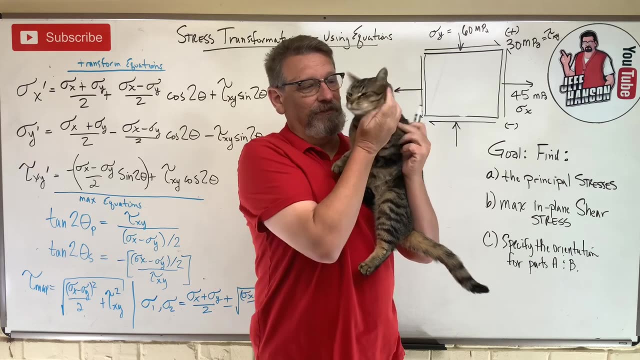 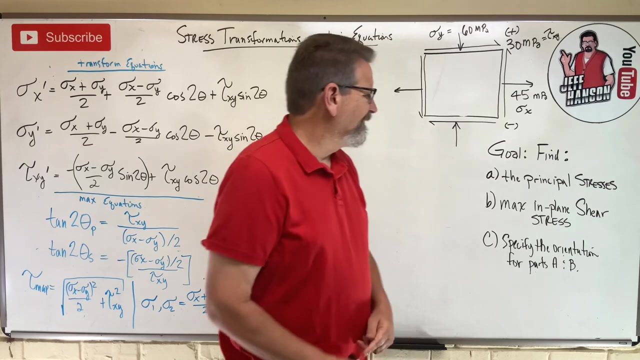 So if I have a stress element as I start to rotate it, then that's wrong. Stripes is stressed out. He needs some help with stress equations too. Do you need stress equation help? Okay, let's go. Okay, you got to go out. Come on, You got to go out. 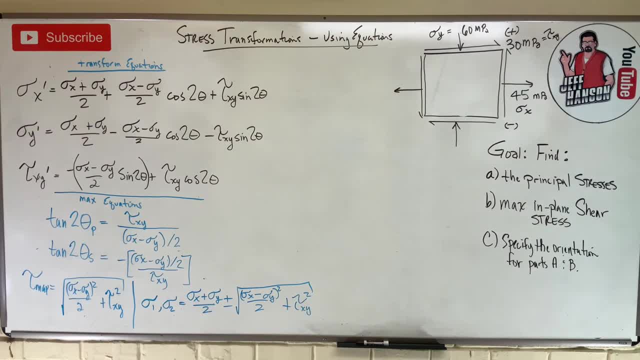 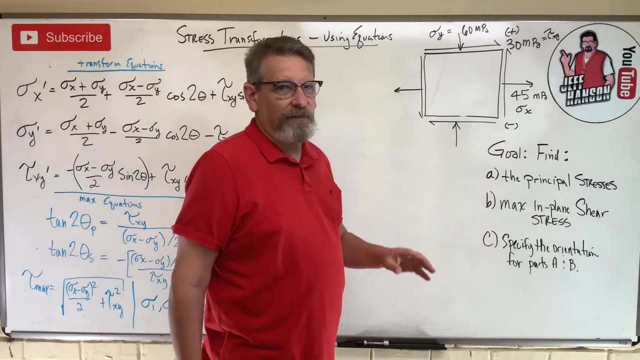 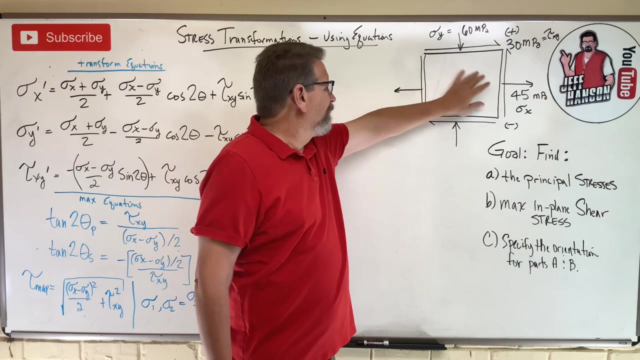 Okay, come on, Okay go. All right, we said stress is directional. So as I start to rotate a stress element, right, These numbers, the normal stresses, and these numbers, the shear stresses, and these numbers, the shear stresses. So, as I start to rotate a stress element, 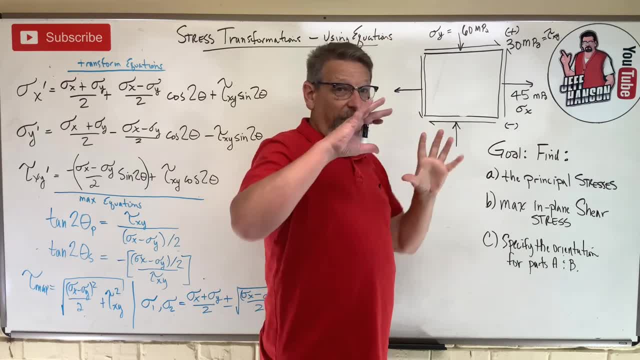 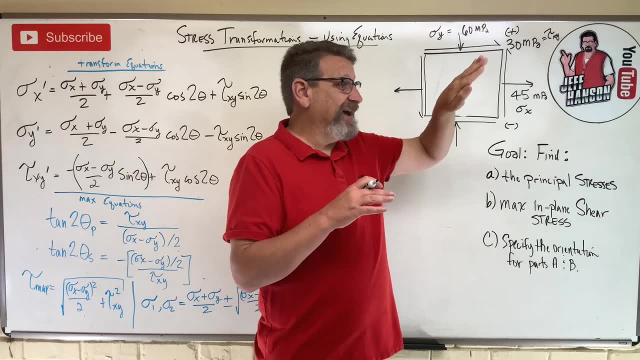 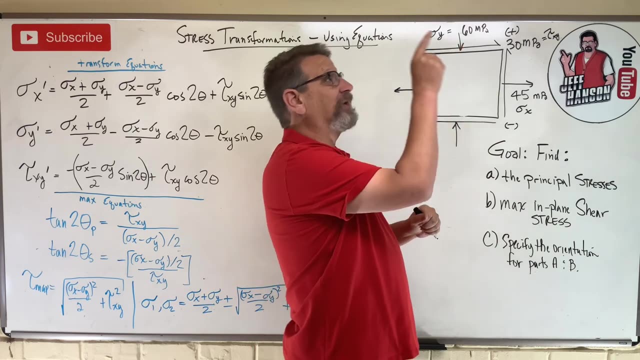 the shear stresses start to change. They'll go up, they'll go down, but what they'll eventually do is they'll go to a maximum place. And then, once they get to a maximum, just think about, like, if I'm going to throw a ball, If I throw it at 45 degrees, I'm going to get maximum If I throw it. 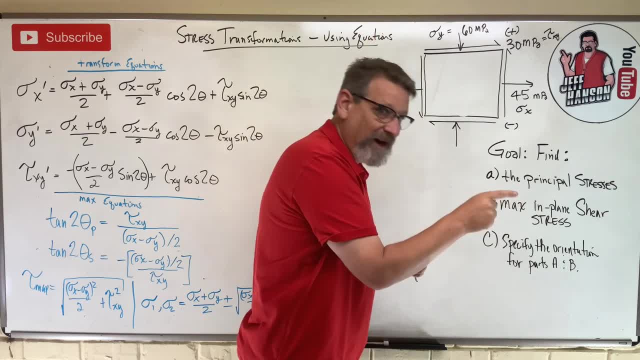 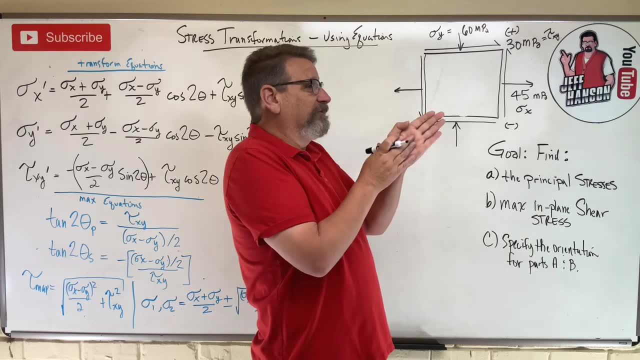 any higher than that, I'm going to get less. If I throw it any lower than that, I'm going to get less distance right. Same thing for stress. Stress is maximum at 45 degrees. So if I go to 45 degrees, 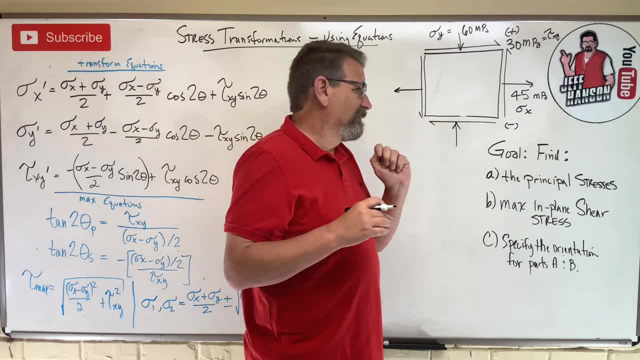 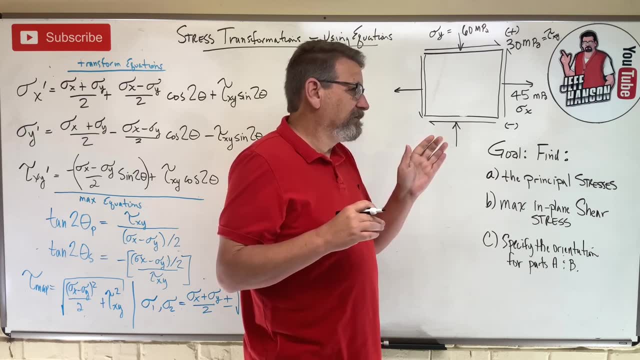 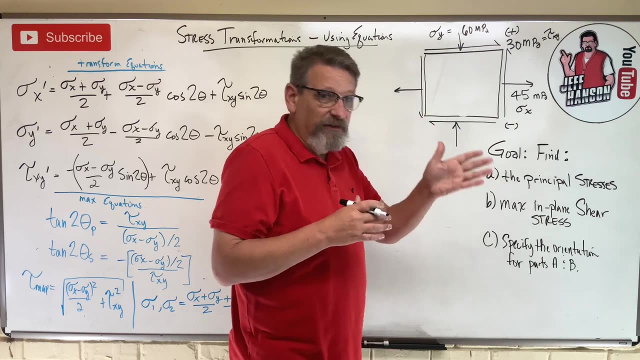 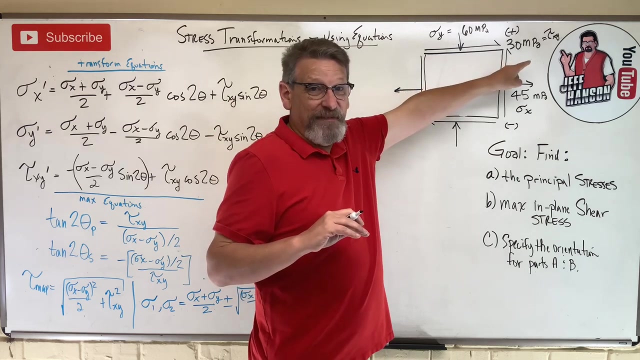 well, that's not true. So same thing for stress, Stress. there is a direction where the normal stress is going to be maximum and there is another direction where shear stress is going to be maximum. okay, So last time we just found out, let's just transform this to some. 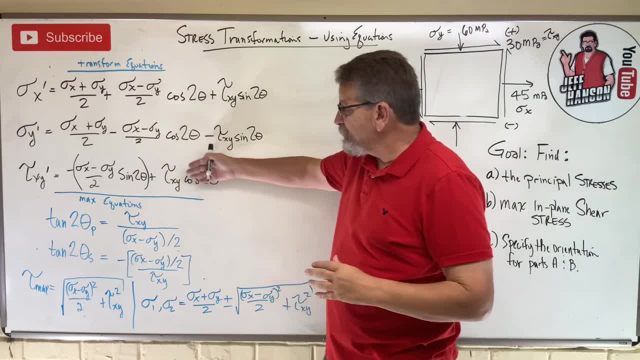 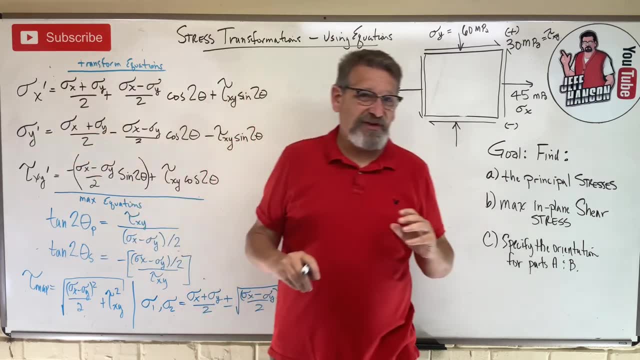 random angle, right, And we can use these equations to transform it to any angle in the world we want, and I'll tell you what the new sigma x is and the new sigma y is okay, But in this lesson we're really focused on finding what are those maximum numbers When? 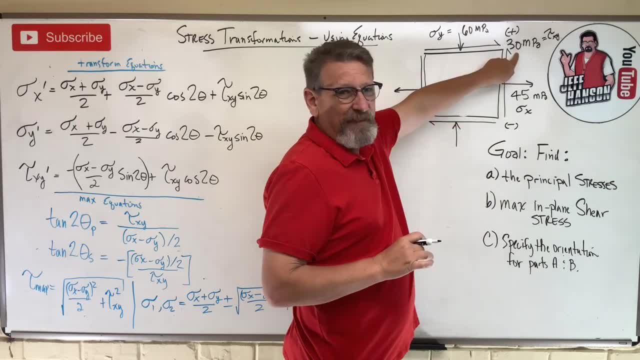 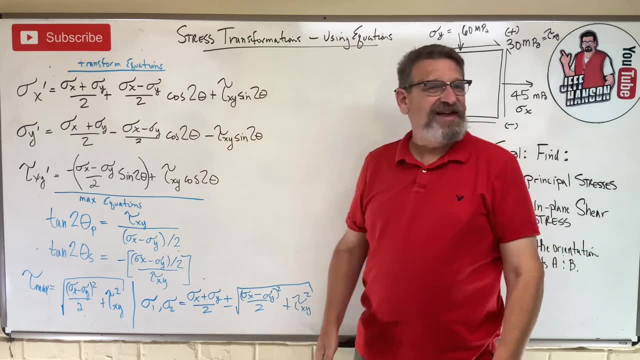 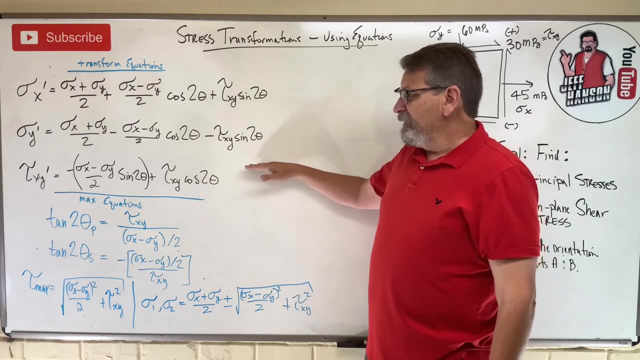 is this maximum? When is that maximum? okay, And we have a new set of equations Again. can I remember all of these equations? Heck, no, I can't remember them. I've been doing this for years. I can't remember this. okay, So there's a better way coming, and it's coming in the next. 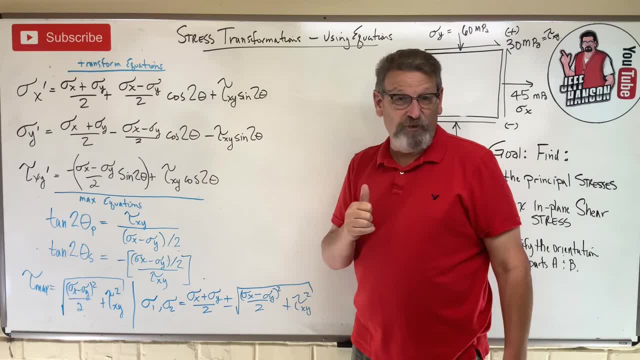 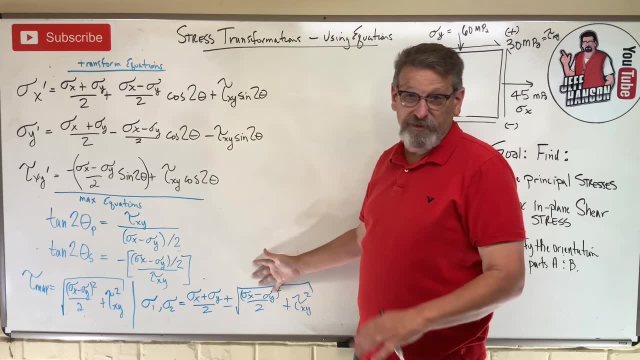 video and it's called Moore's Circle. It's a graphic method That I can remember. I can get these same numbers using that method, so you don't have to use this. But for some reason, Johnny Weeksauce, the super student, wants to use equations because some professors- I being one of- 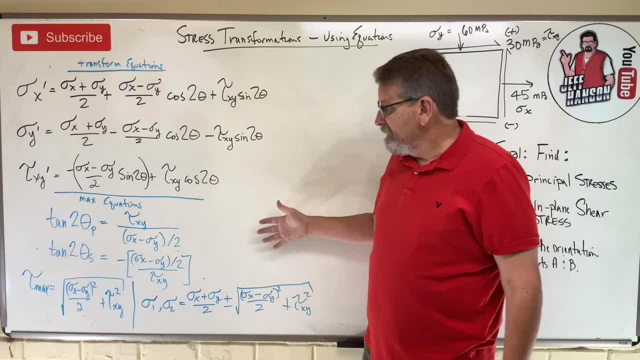 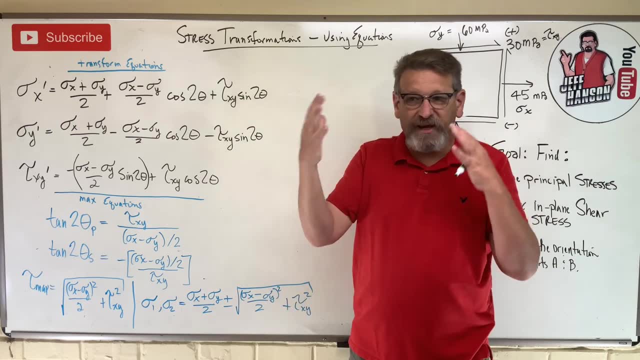 those will let my students have an equation sheet- the one in the front of the book- and if you're allowed to do that, then you have these equations and it's just a matter of plug and chug. But I don't think you get a physical understanding about what's really going on. so 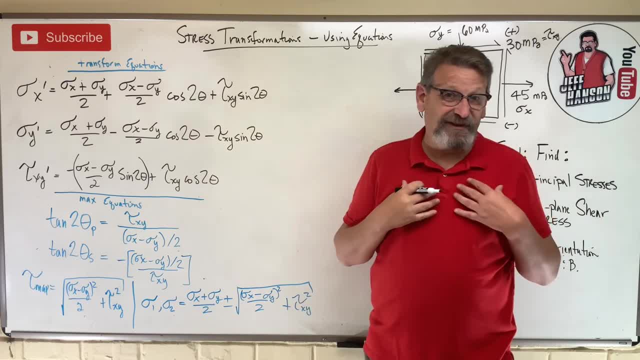 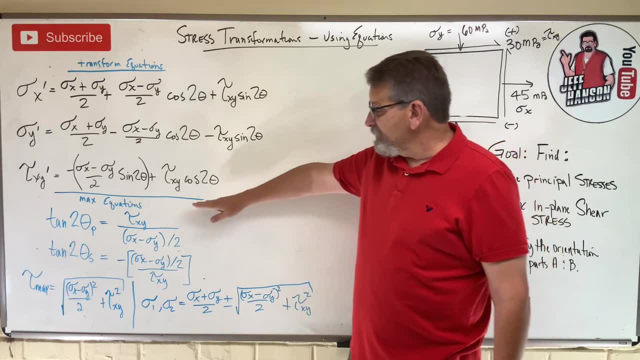 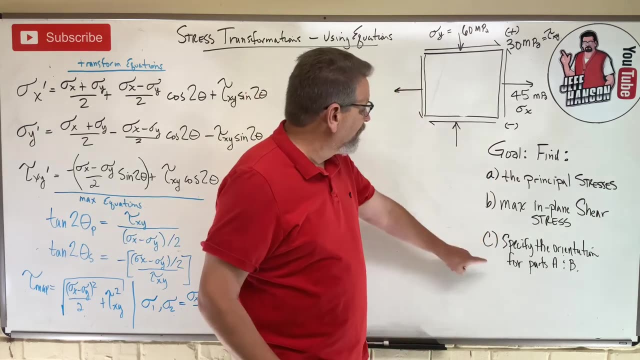 not a fan of using the equations. Personally, I hate it. I wish that you know I've been dreading making this video, but here we are. okay. So the maximum of equations, The first two here, are to find theta p and theta s. Now we're going to need those down here. on part c when it says: 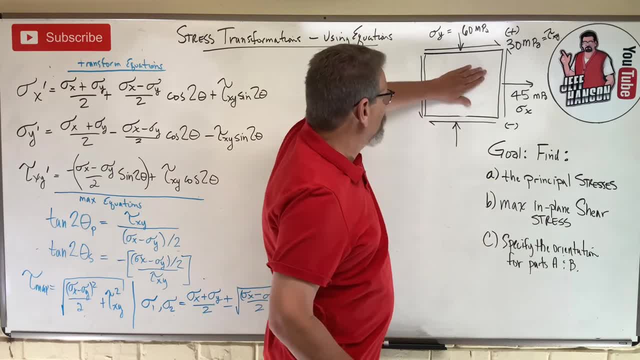 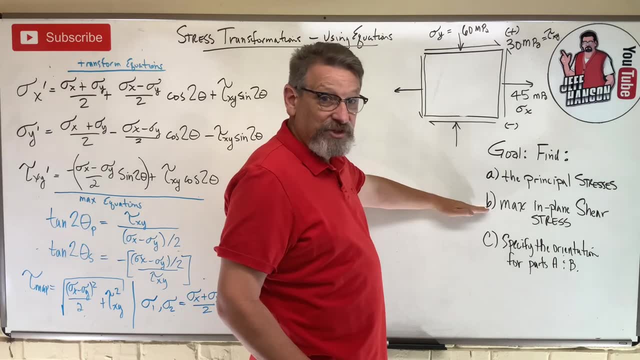 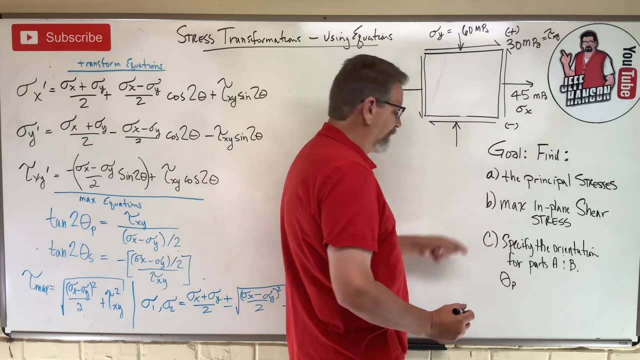 specify the orientation. So what is the orientation of the stress element? to find the principal stresses. What is the orientation of the element to find maximum shear stresses? Those two orientations are called theta p, that's for principal stresses, and theta s, that's an s. 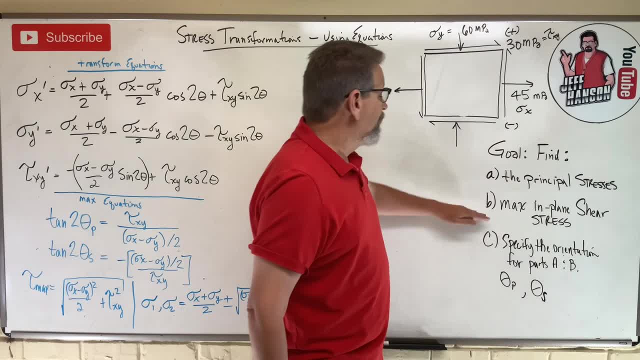 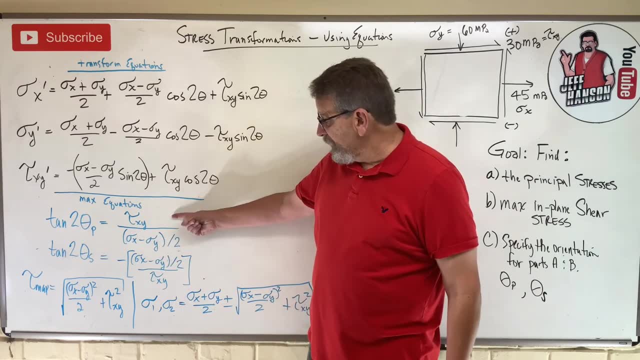 not a five, an s for maximum shear stress angles. okay, And I'm going to show you how to find those angles. Well, there's the equations right there. Notice that this equation and this equation are the same, except for the second one. So the first one is theta p and the second one is theta s. 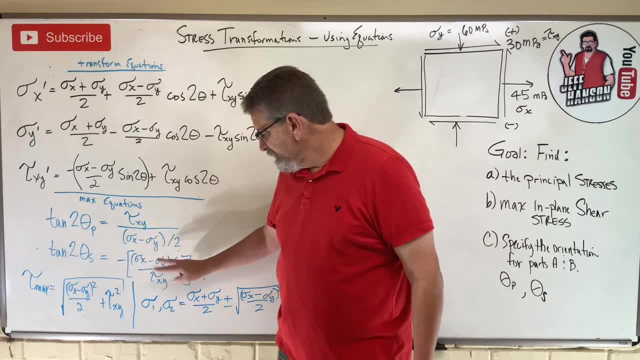 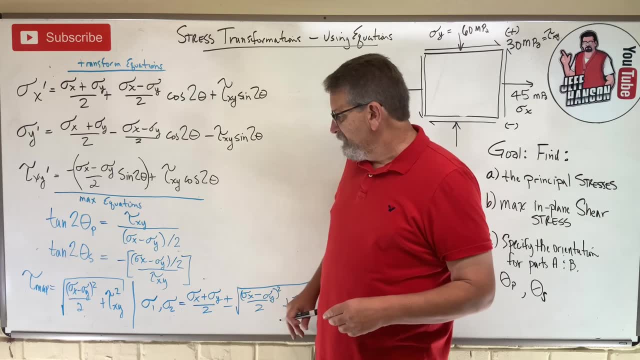 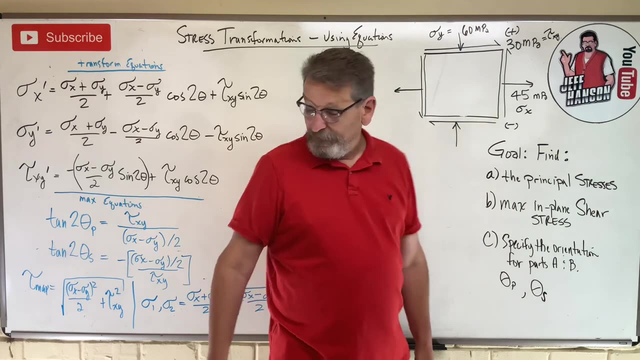 The second one here, the shear stress, is the negative inverse. This whole thing is just flipped over, isn't it? Same equation, but the negative inverse. okay, Then here's an equation to find tau max, that is, maximum shear stress. That's the equation to find it right there, okay, And then? 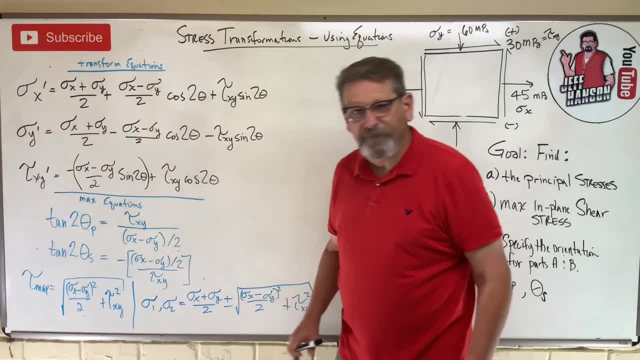 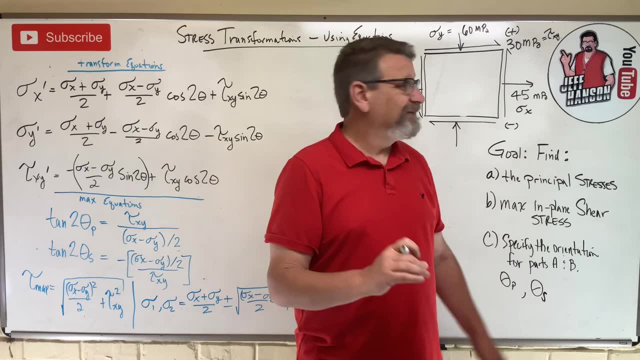 kind of stuck beside him over here. this long equation here on the bottom. That's the equation to find the principal stresses, That is the maximum shear stress. That's the equation to find the maximum and the minimum stresses, that this can be Maximum, minimum right Or maximum minimum. 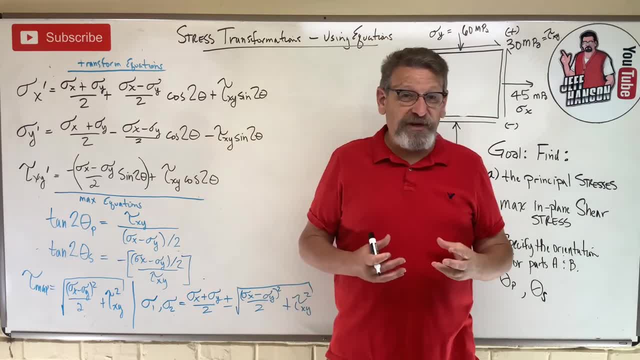 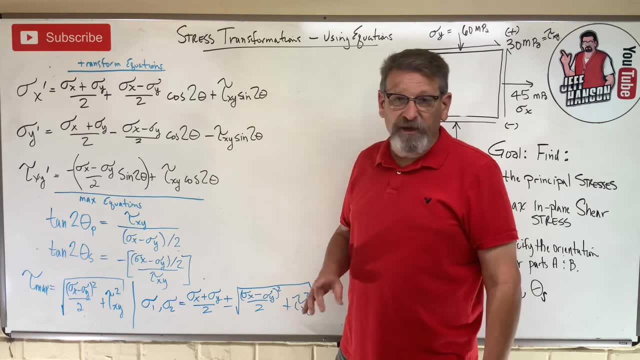 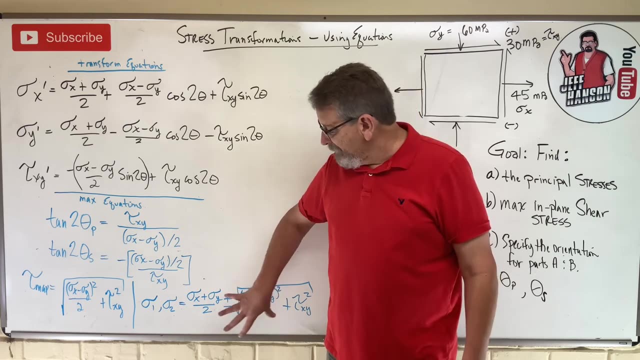 And we call those theta one, theta two. So those principal stresses are called theta one and theta two. okay, Now there's a couple of nuggets here. Number one: when I am at principal stress. this is always, always okay When I am at principal stress. 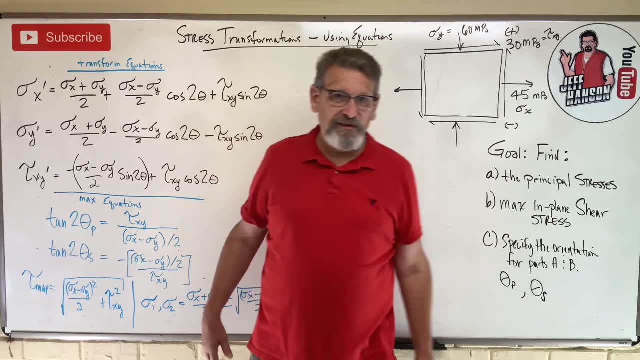 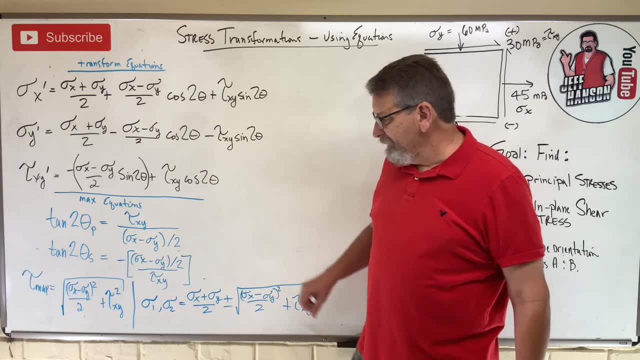 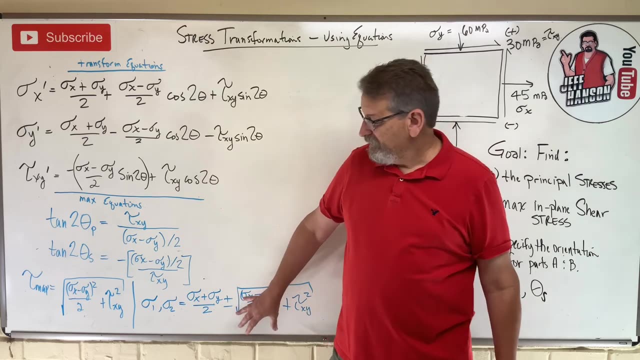 it will be equal to zero, always okay. So when I find these guys that one is zero okay When I'm at that guy, then normal stress: maybe he's zero. No, he's not zero When I'm at tau max. 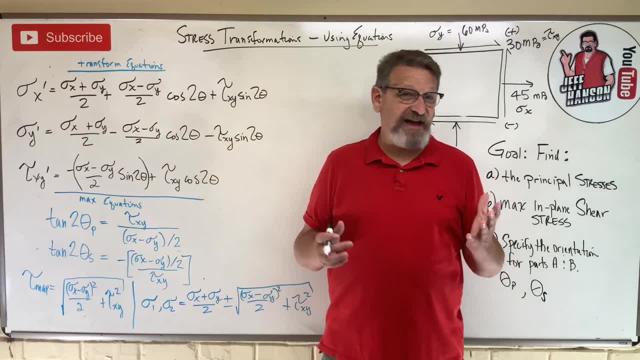 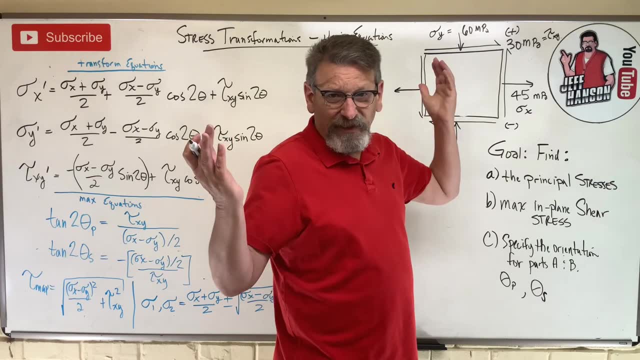 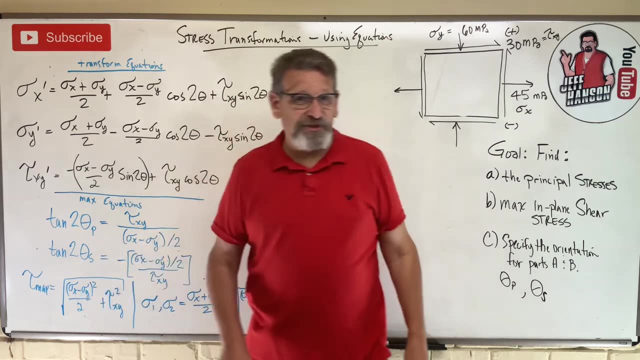 normal stress is called sigma average. Now, sigma average is pretty easy to find. It's that plus that, Divided by two. right, That's sigma average. okay, And when you're here, sigma average, your stress element, this one and this one will be exactly the same. It's sigma average. This is 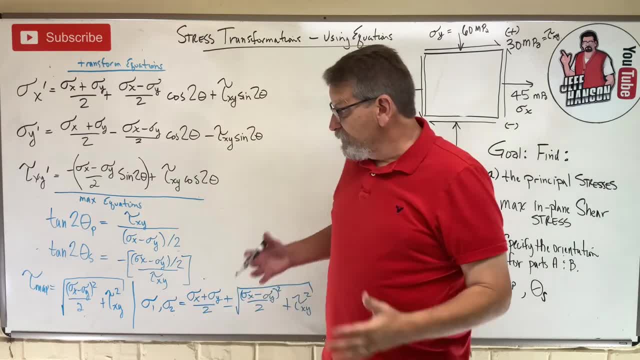 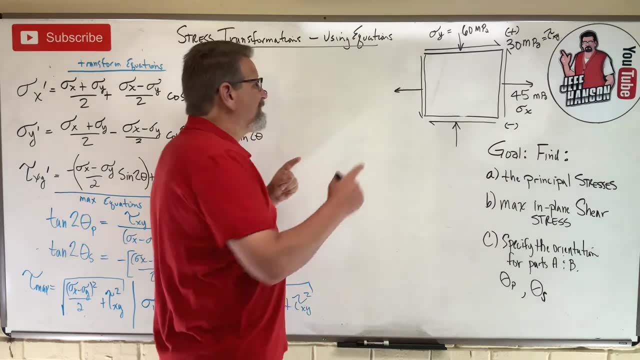 the same as that. They're both average value, okay. So there's a couple of little secret, little nuggets. Let me give you one more little pro tip. okay, We've been kind of going on. we've been talking about this guy right here, tau xy. Have you ever seen that? 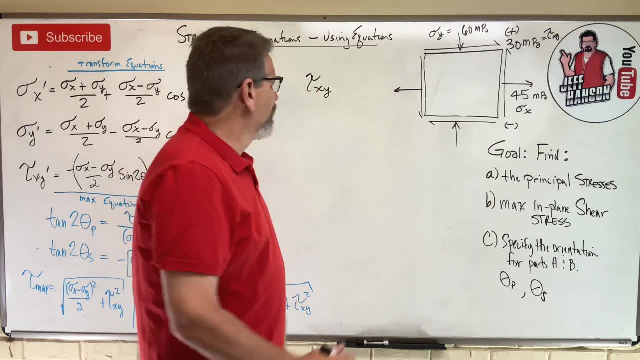 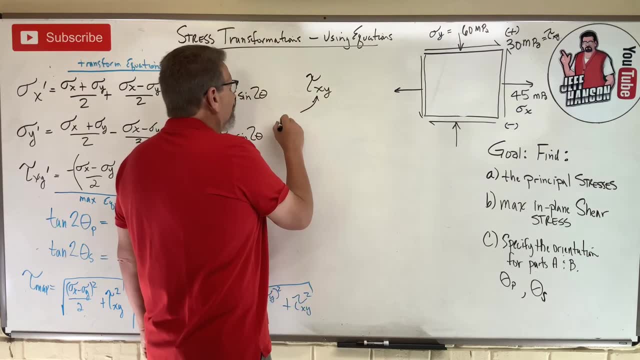 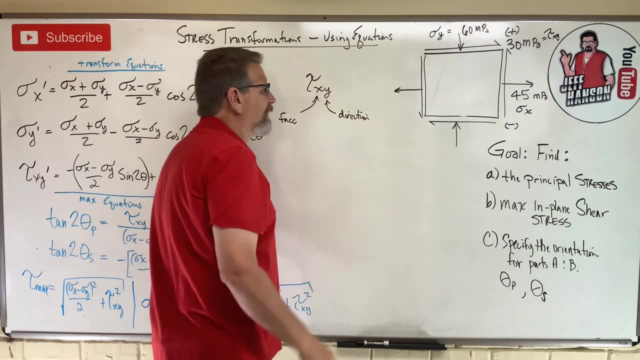 And you're wondering: why do they call it xy? Here's the little secret nugget. This is a little secret decoder ring. This is only for the pros, okay, Amateurs, tune out. X is the face, okay And y is the direction, okay. So when I'm talking about this guy right here, this vector right here, 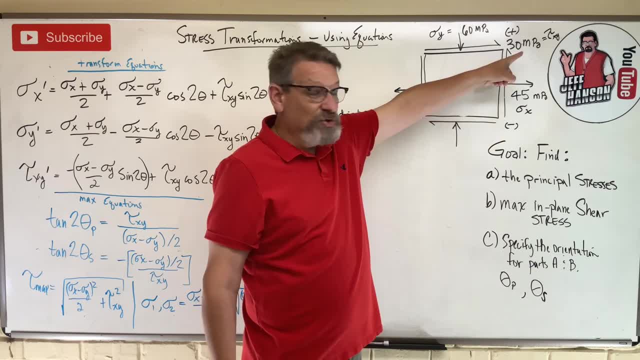 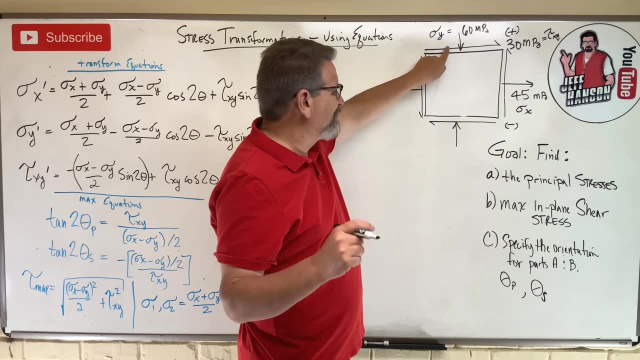 it's on the x face and it's pointed in the y direction, So I have tau xy. So what would this guy right here be called? He's on the y face, He's in the x direction, So that would be tau yx. right, Then you can have tau xz, tau yz. 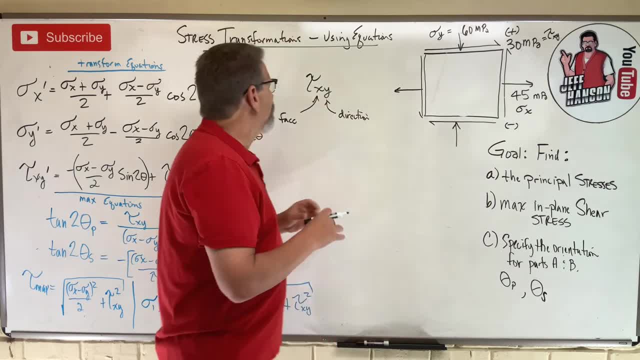 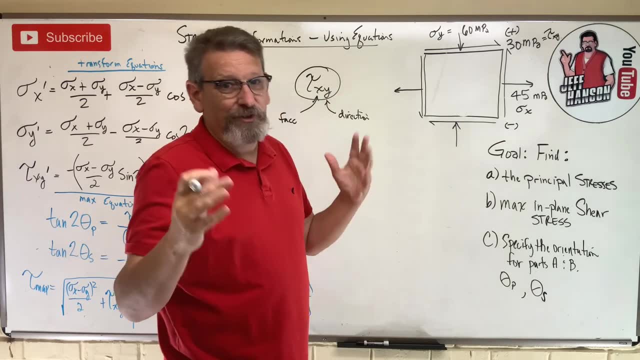 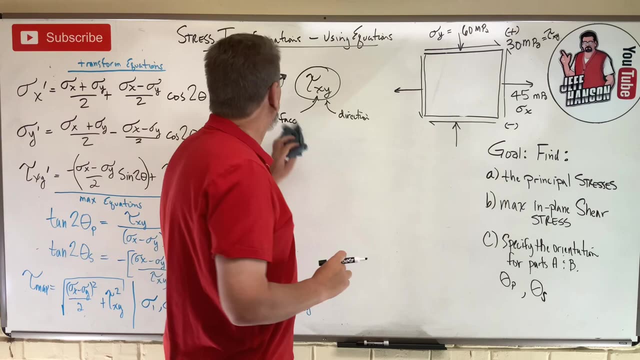 tau zy. right, You can get all kinds of different ones, But that little notation, this little notation right there, that's the face, that's the direction, There's your little secret nugget of the day, Okay. So, with that behind us, okay, With that behind us, let's. 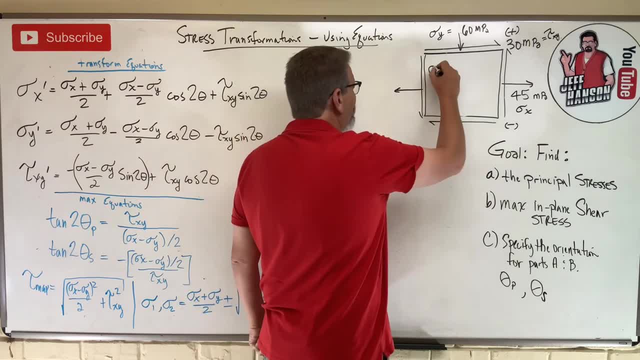 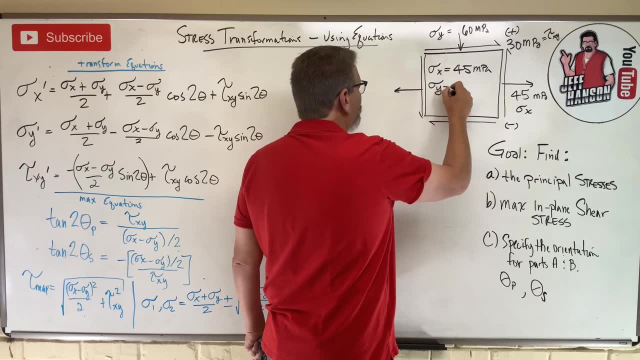 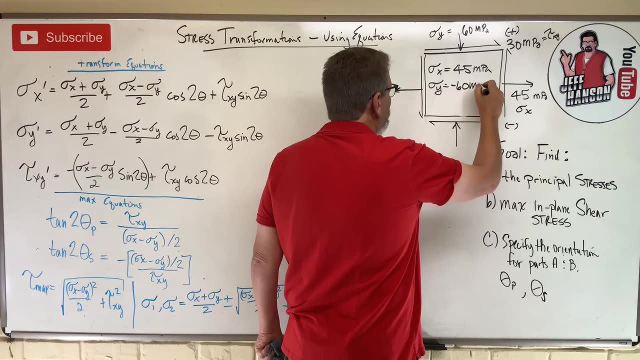 start going over here. Now, what I've got here is this: Sigma x is equal to 45 megapascals. Sigma y is equal to look it's in compression. What does that mean? It's negative, okay. And then, of course, tau xy. 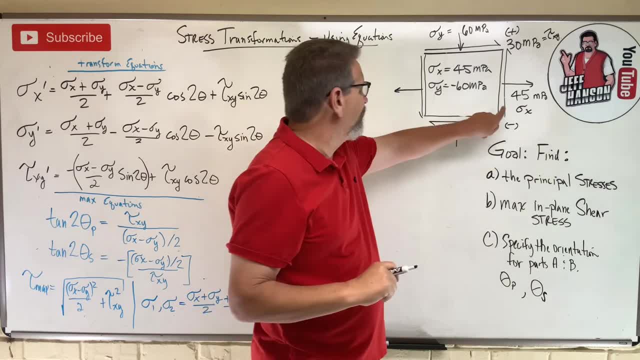 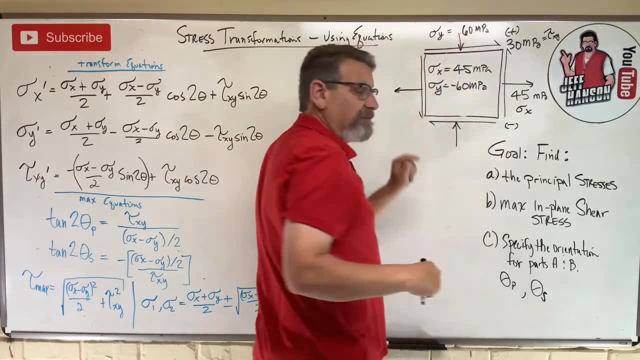 Now we got to tell if that's positive or negative. We always look at the x face. And which direction does this arrow rotate? my little stress element That's going this way. That's rotating me, Okay, Counterclockwise. Counterclockwise is positive, isn't it? So that's going to be. 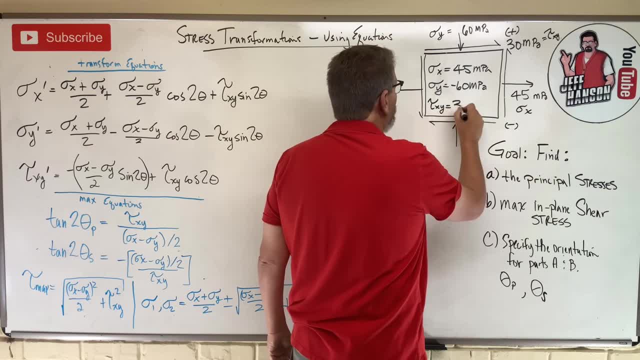 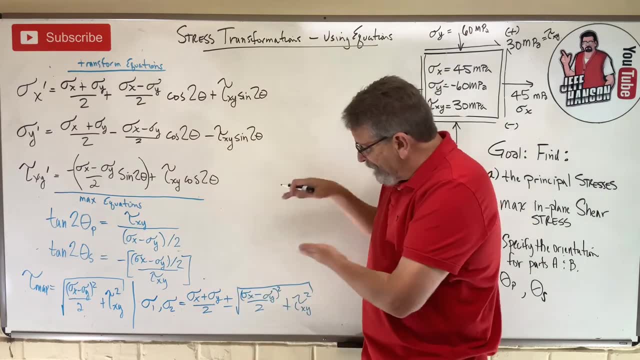 so tau xy is equal to positive 30 megapascals. okay, So there's our three numbers that are going to go into bam bam, those equations down there. okay, So let's just start off with part a. 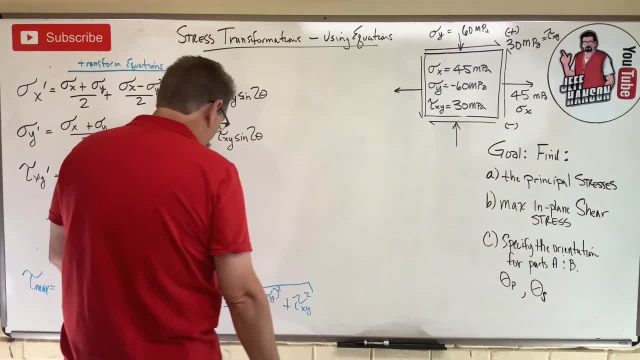 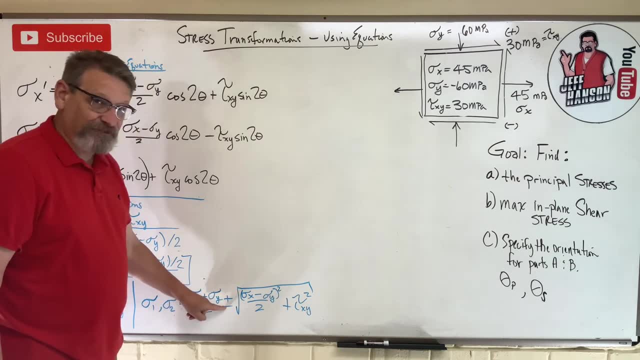 What are the principal stresses? All right, We're going to use this jumbo equation down here And notice what you've got: Sigma x plus sigma y divided by two, And then plus, minus. The plus is going to be sigma one, The minus is going to be sigma two. 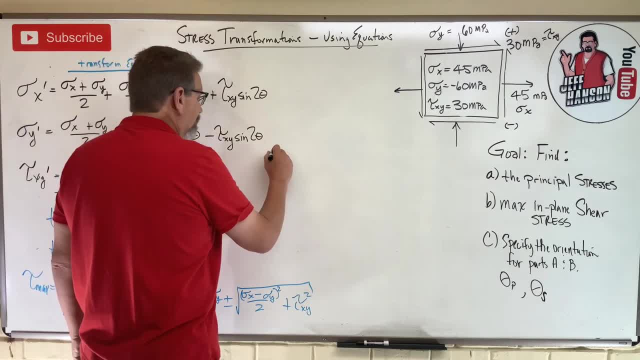 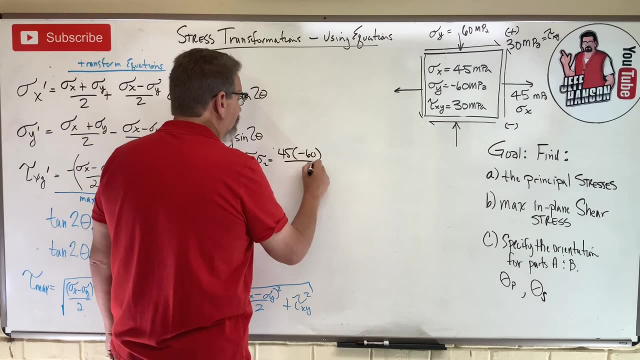 That's it okay. So let's do it right quick and let's see if we can find that. So sigma one, sigma two is equal to right. sigma x: 45, plus sigma y, minus 60, divided by two. 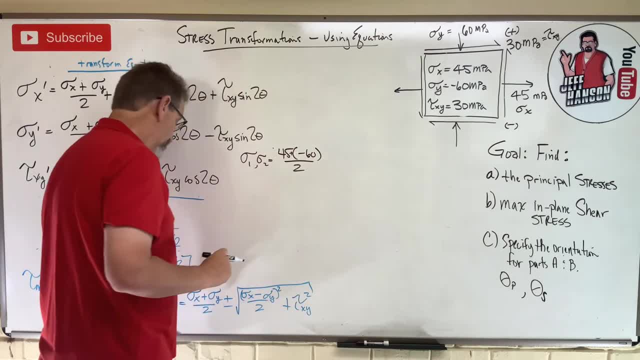 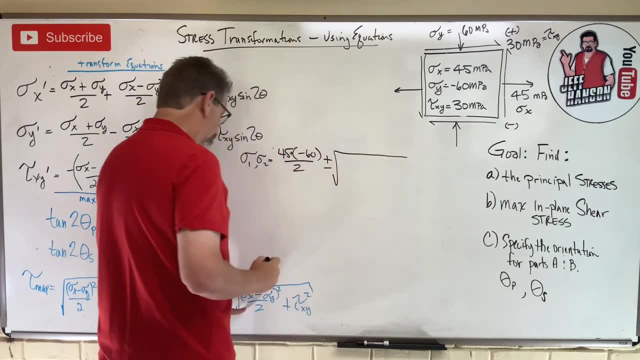 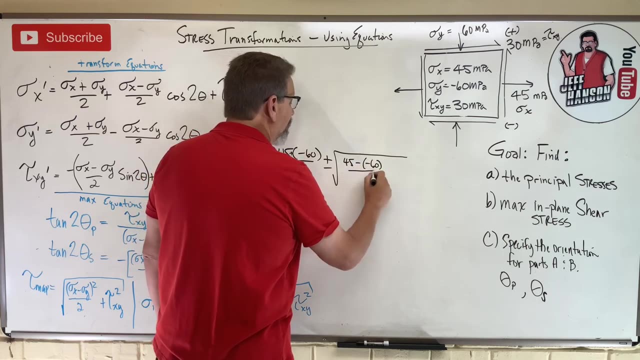 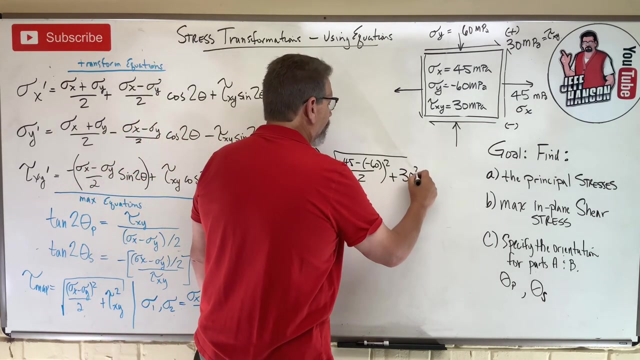 Let's put minus, Sorry, plus there, rather Okay. And then plus minus square root of sigma x minus sigma y, So 45 minus minus 60, divided by two, quantity squared plus tau xy squared. Okay, right, Okay, calculator, what do you got for me here today? 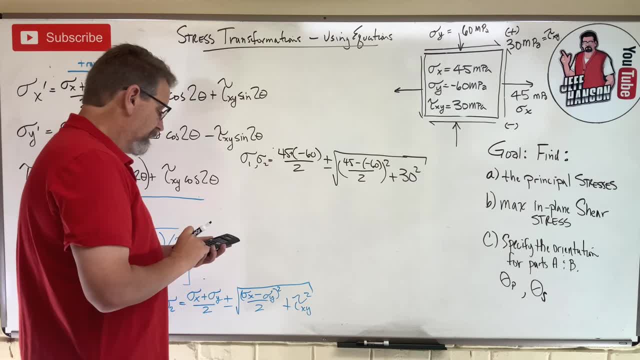 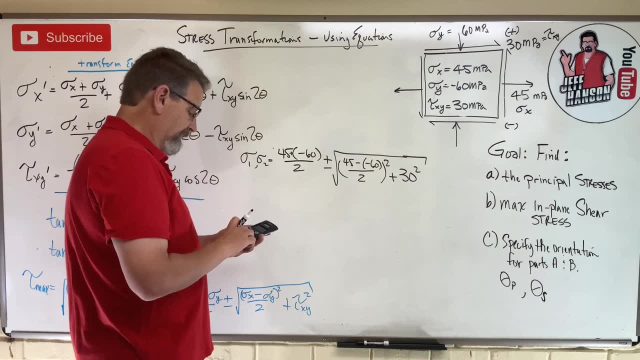 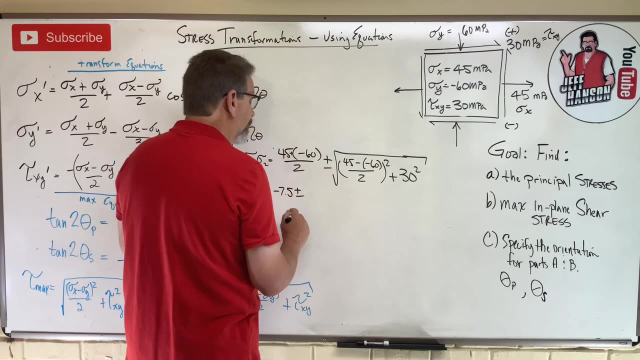 On. I can't turn it on today. There it goes. Okay, 45 minus 60.. 45 minus 60 equals divided by two, equals negative, 7.5, plus or minus. what do we got over here The square root? 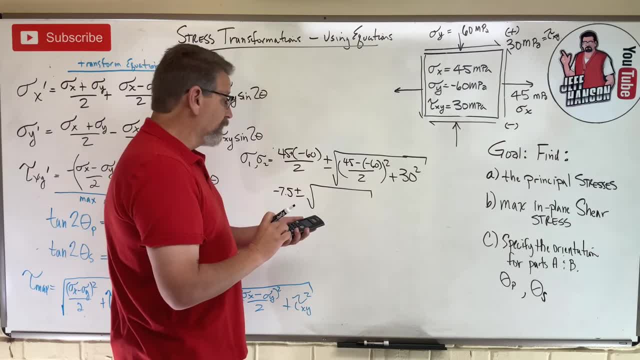 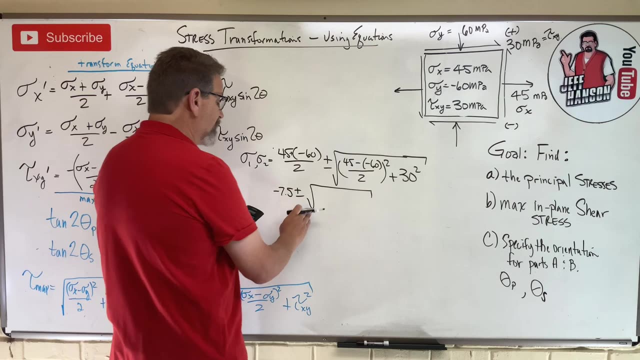 of minus, of minus, turns into a positive. So that's what: 105 divided by two, 105 divided by two equals, and then squared right plus 30 squared equals 36, 56.25.. And then I'm going to square. 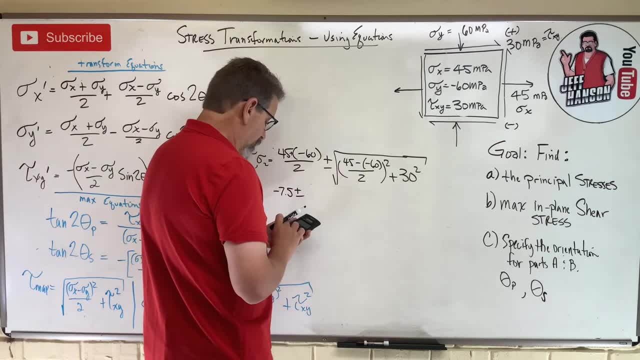 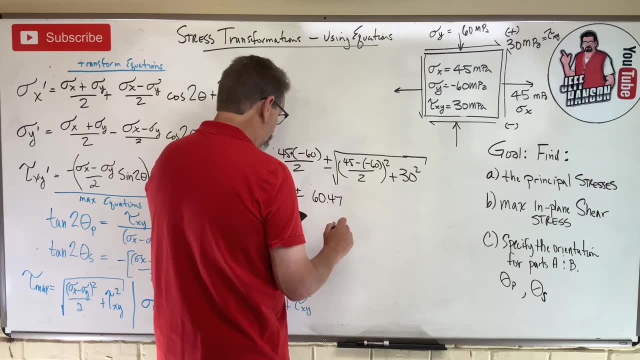 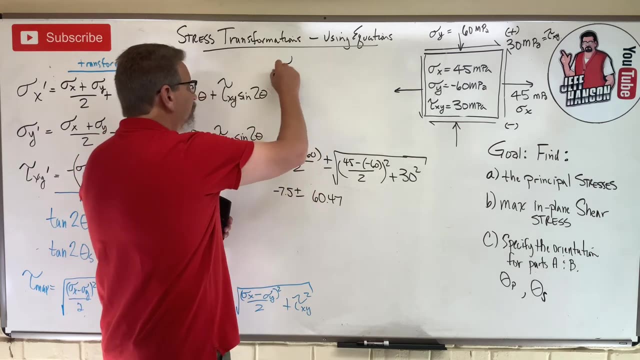 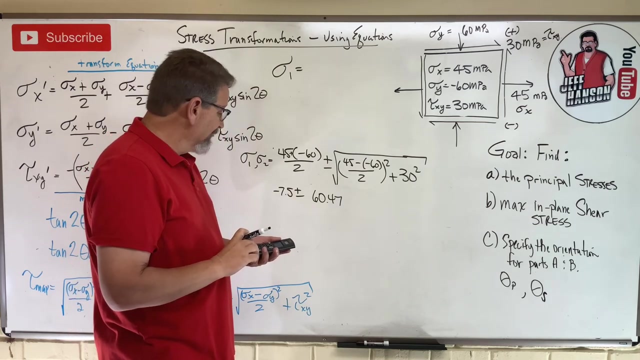 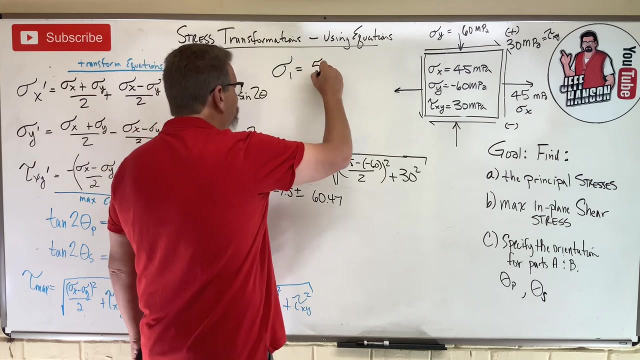 root that right, Second square root, second answer, equals 60.47.. Okay, So here we go. So from this, this is sigma one. sigma two, we get this Sigma one. the principal stress is equal to what: 60.46 minus 7.5.. 52.96.. Let's call it 53,, shall we? 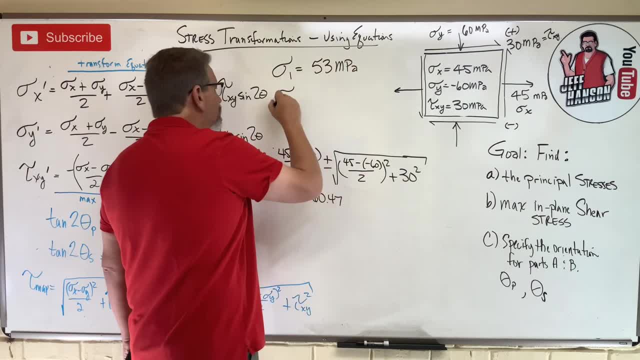 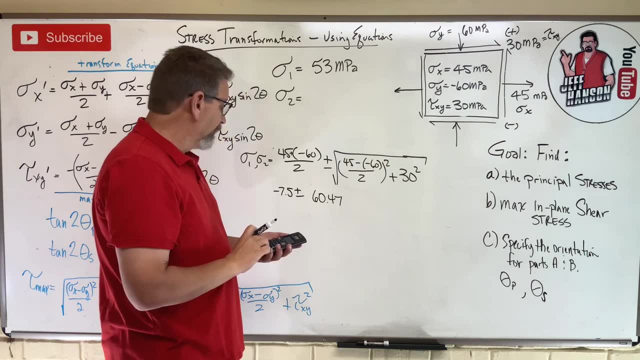 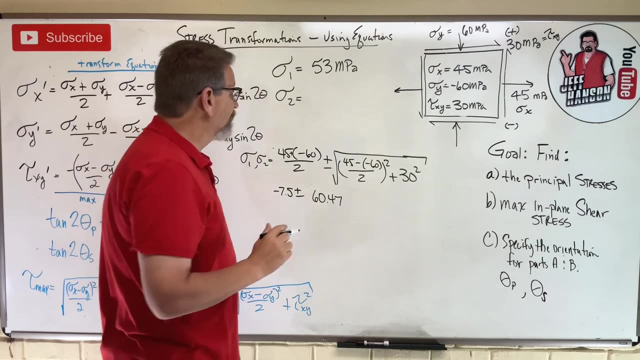 Okay, Sigma two is equal to 7.5 plus 60.47.. Okay, Sigma two is equal to 7.5 plus 60.47.. Okay, Sigma two is equal to 7.5 plus 60.47.. Let's call it negative 68. Okay. 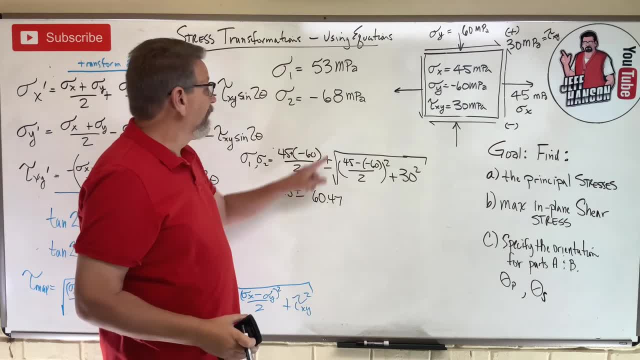 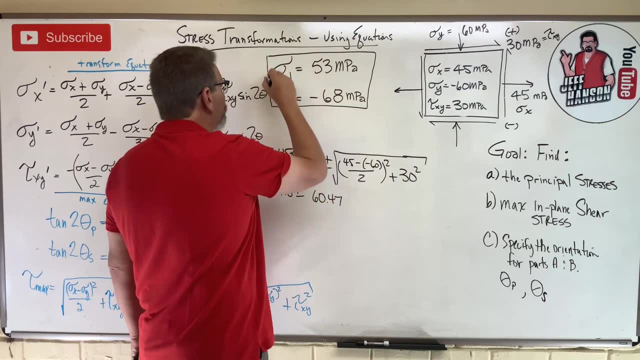 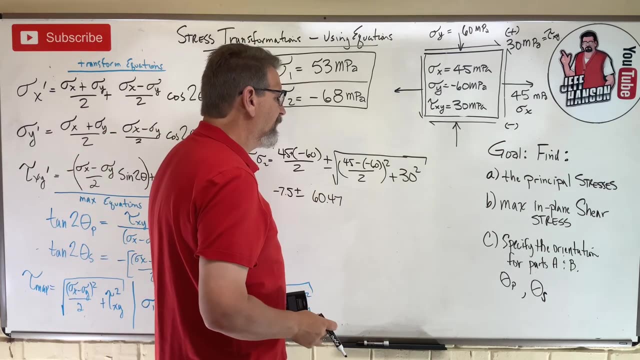 You with me on that Minus and a minus make a big minus, right, That guy? Okay, So there's sigma one and sigma two. our principal stresses, And that's how you find those Okay. Now, now that I have those, okay, let's well, let's find the next thing, Let's find maximum. 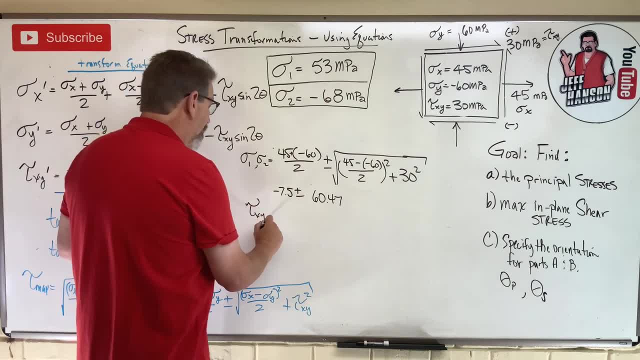 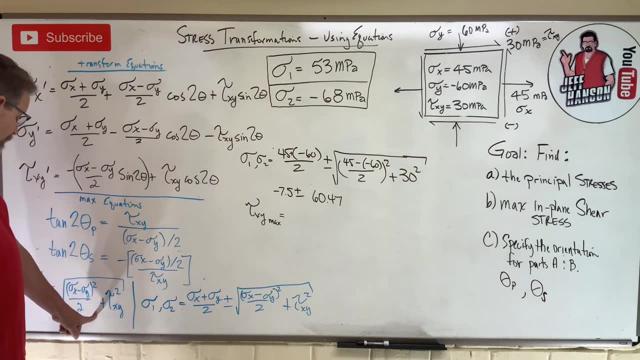 input. Okay, So let's find the next thing, Let's find the next thing, Let's find the next thing. Alright, So let's reach the end, the next table, do that, and then we're gonna do three. 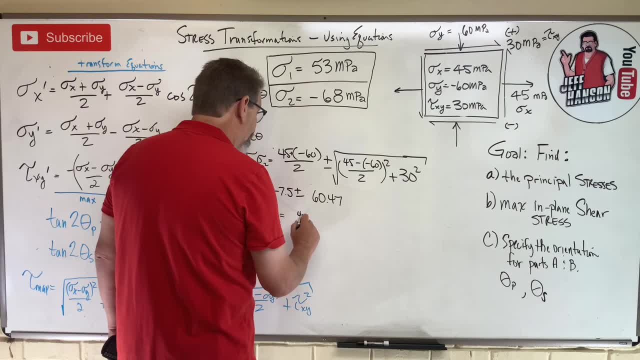 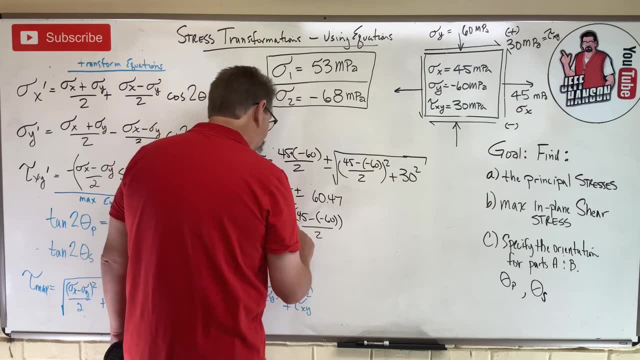 numbers. three add-ons. we'll do them in two. we're gonna do three add-ons in two First. all right, Now we're gonna write everything, all right. So we're Till nuts these twin towers. Yeah, Let's get the violet. 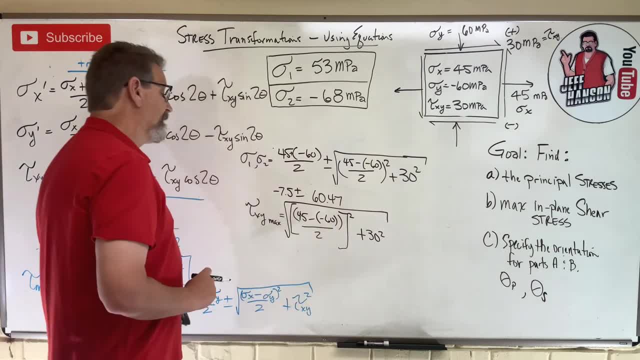 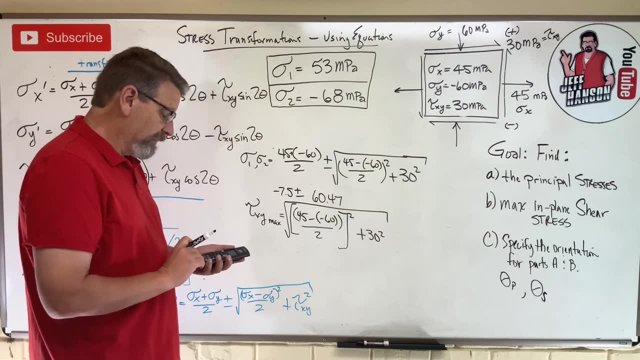 Okay, square root. okay, What's that going to be? So that's again: 105 divided by 2, 105 divided by 2 equals you know what it's going to be. This right here and that right there is the same It's going. 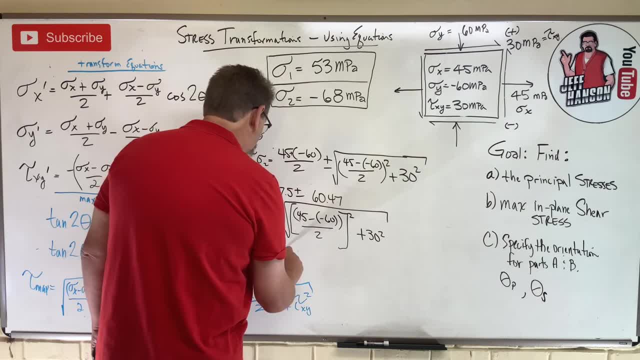 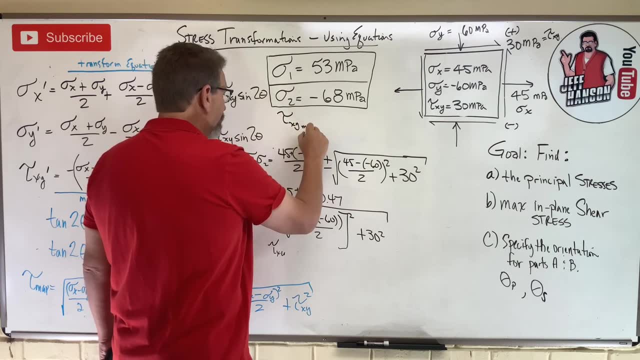 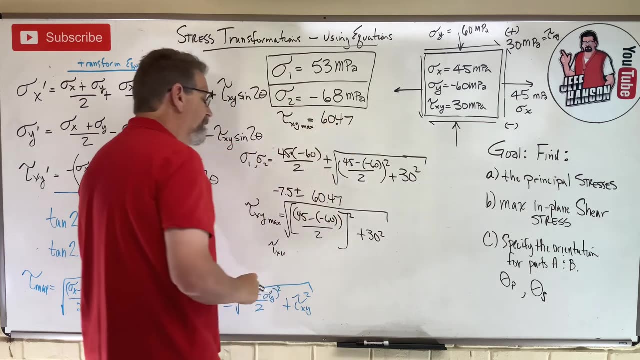 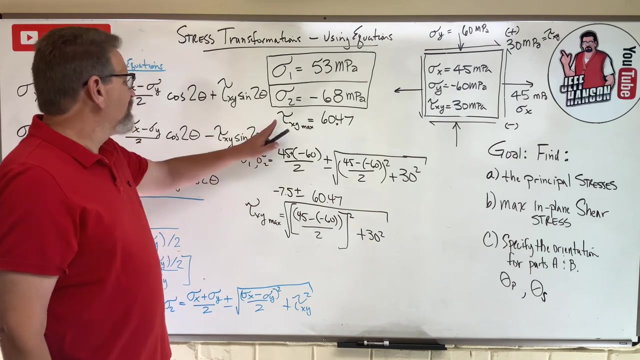 to be 60.47,, isn't it? Tau x y? well, let's write it up here: Tau x y max is equal to 60.47,. okay, There you go. Are you with me on that? So far, so good. We see how to calculate those guys. 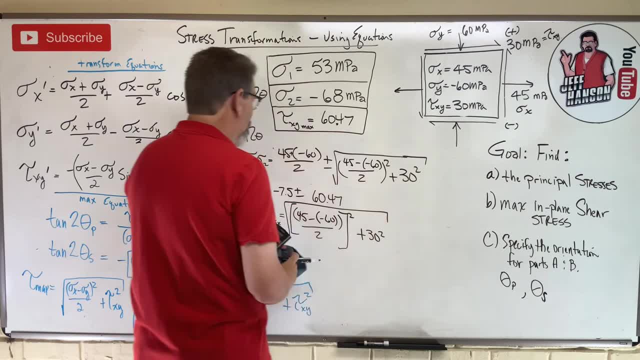 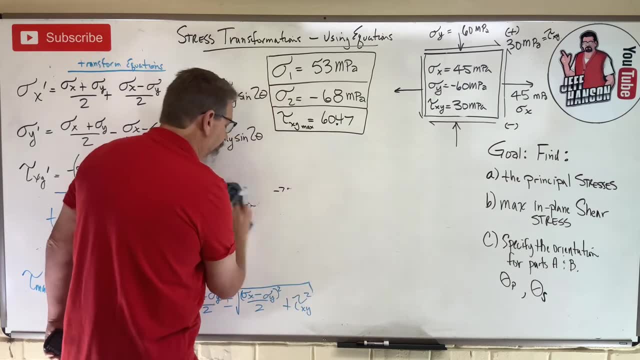 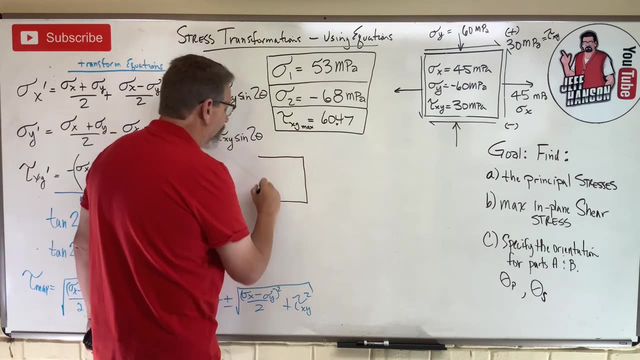 right. So that's part A and part B. Now let's do this. Let's clear up a little more confusion, okay, And let's draw a stress element. okay, Number one: I'm going to draw a stress element for principal stress. 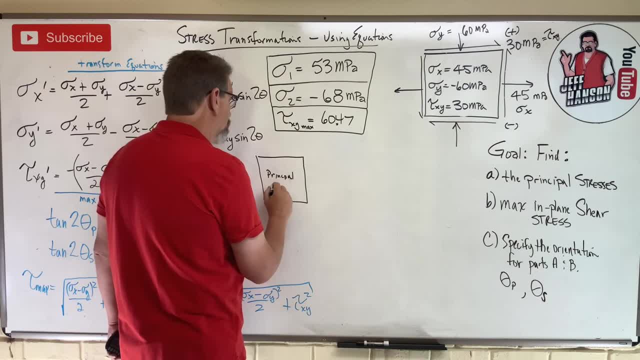 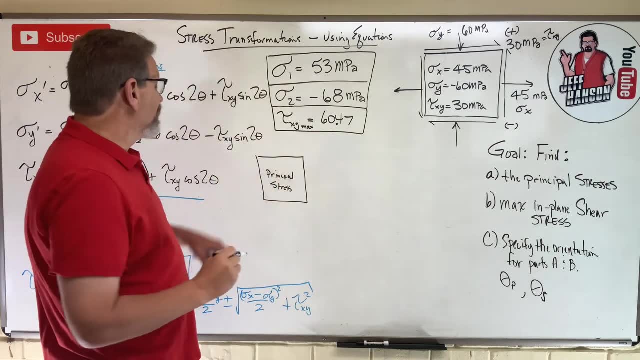 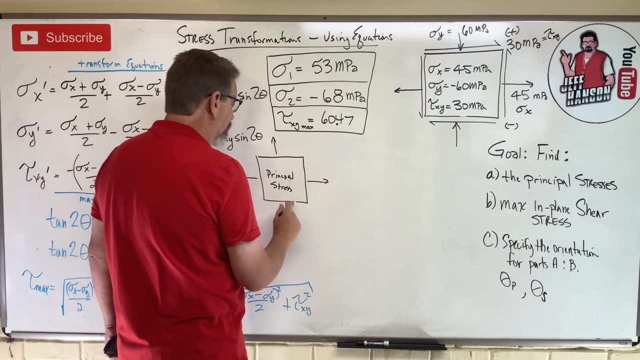 Is it L-E or A-L? I don't know. okay, I think it's A-L. Here we go. Sigma 1 is sigma 2.. Okay, Here's my new stress element. Well, one of them's going to be negative, isn't it? 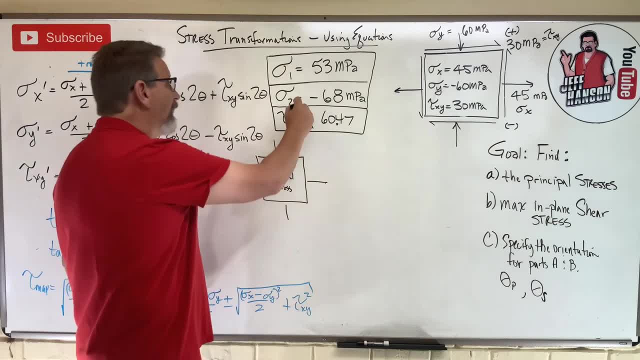 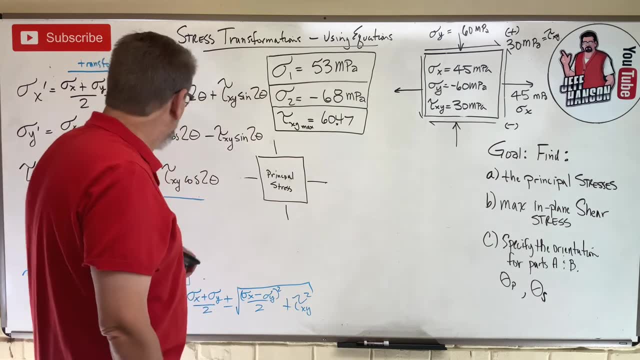 How do I know which one sigma x is and which one's sigma y? Because I just got a 1 and 2.. How do I know which one to put on the x face, which one to put on the y face? Well, I'll tell you how to do. 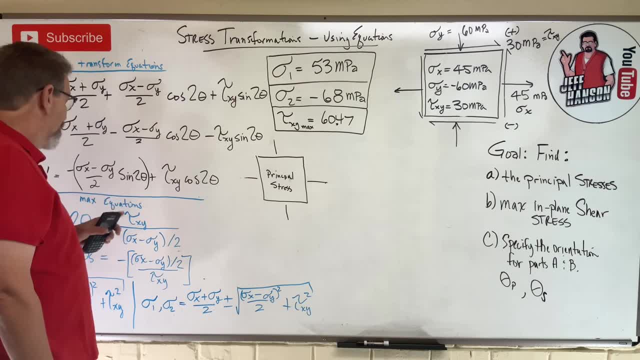 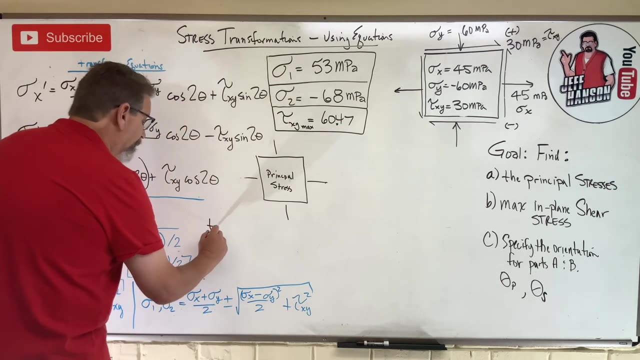 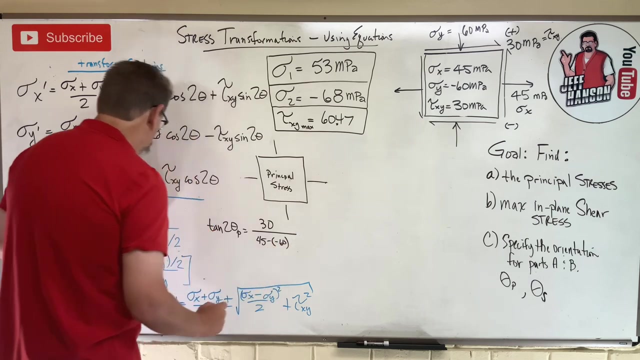 that, And as soon as we do one more thing, and we find, let's find that orientation for the principal stress, is this top equation here right? Which is what? Tan 2, theta p is equal to tau x, y, 30 divided by sigma x minus sigma y, 45 minus minus 60 divided by 2, okay, So again, that's 105 divided. 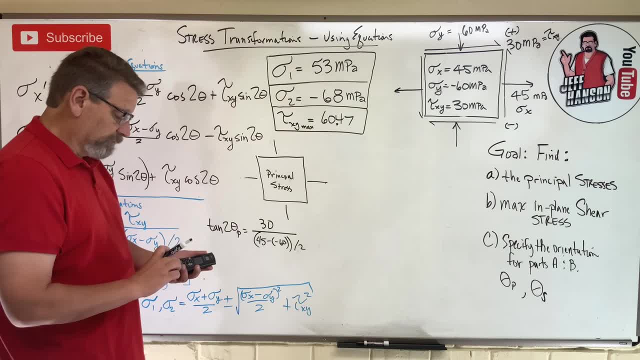 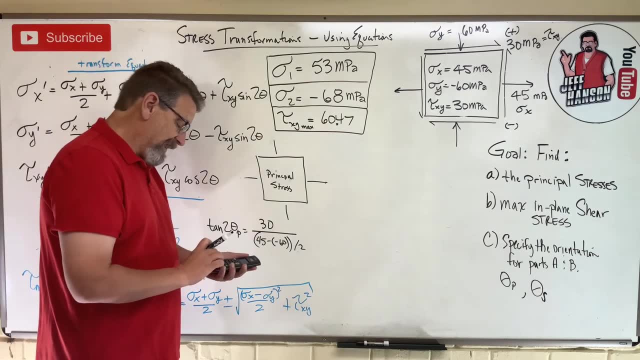 by 2, 105 divided by 2 equal. Okay, So again, that's: 105 divided by 2, 105 divided by 2 equals. Oh clear, 105 divided by 2 equals 52.5, and then 30 divided by that. 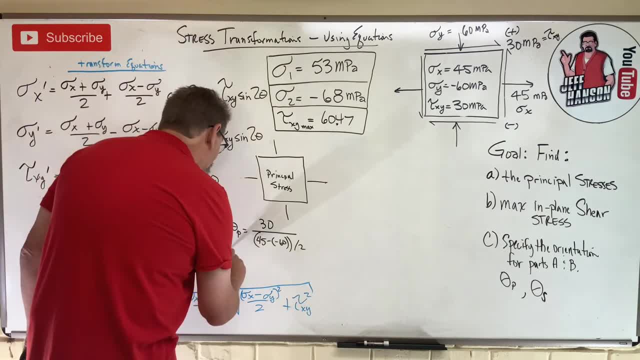 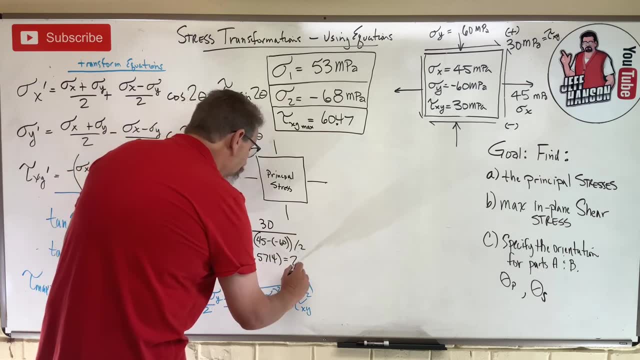 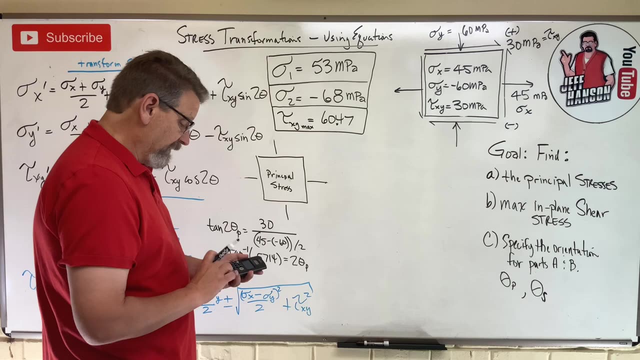 0.5714.. So tan inverse of 0.5714 is equal to 2 theta p, right? So I'm going to inverse tan that Second answer equals. So I got 29 degrees and then I'm going to. 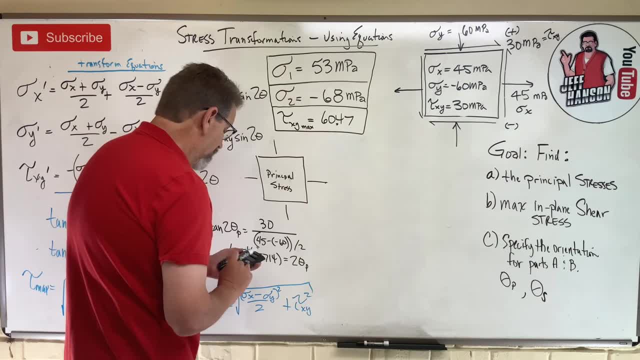 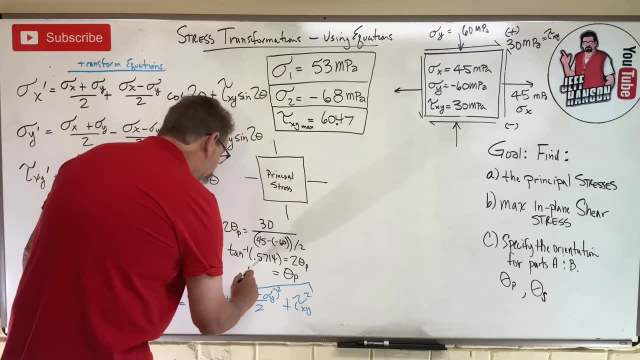 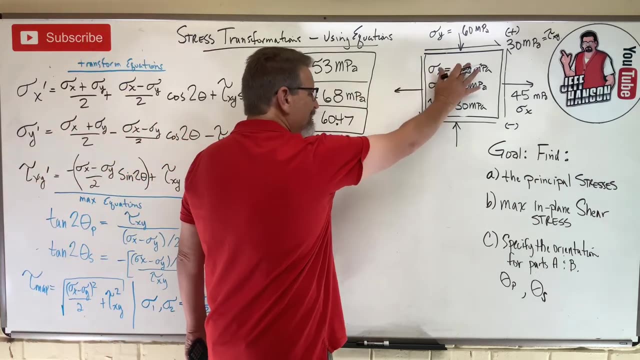 divide that by 2,, divided by 2, and I get this- theta p is equal to 14.87,. okay, So what does that say? That says I need to take that stress element and rotate it. Now I got a positive 14.87,. 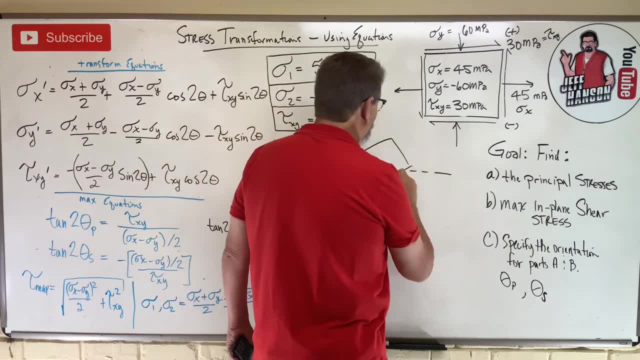 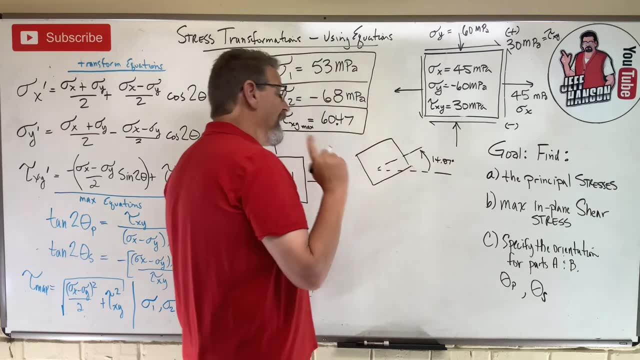 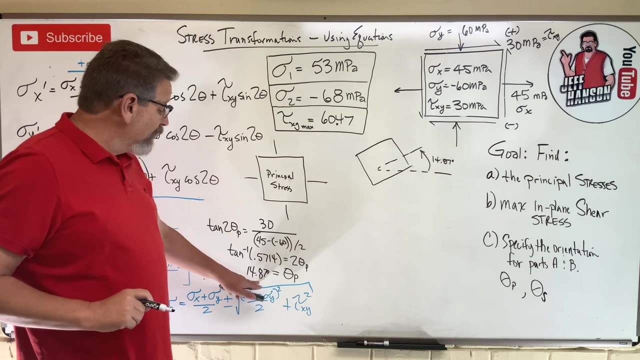 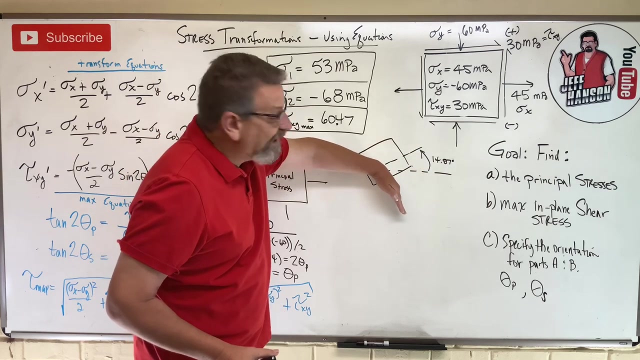 so what does that mean? That I'm going to rotate it in the positive direction. That is this way: whoop, 14.87 degrees. okay. Now it's also acceptable and actually proper to have two angles on this, because I can get to the principal stresses by rotating this way or by rotating that. 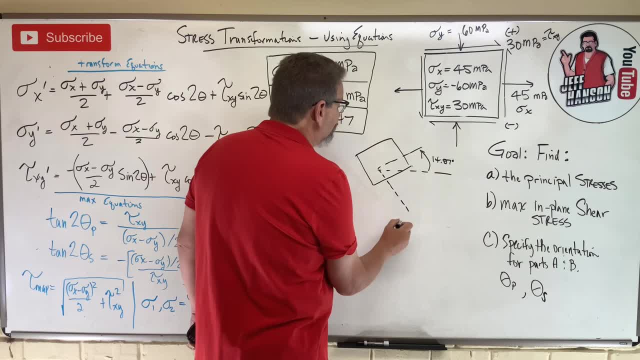 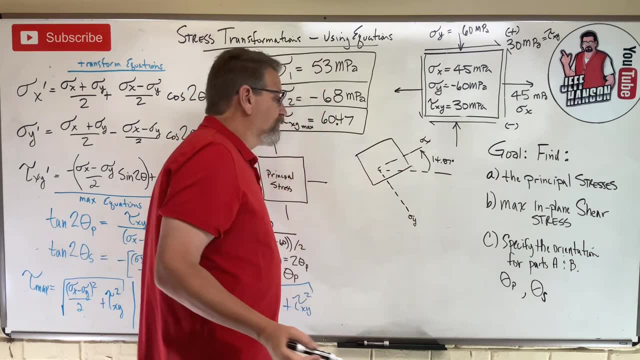 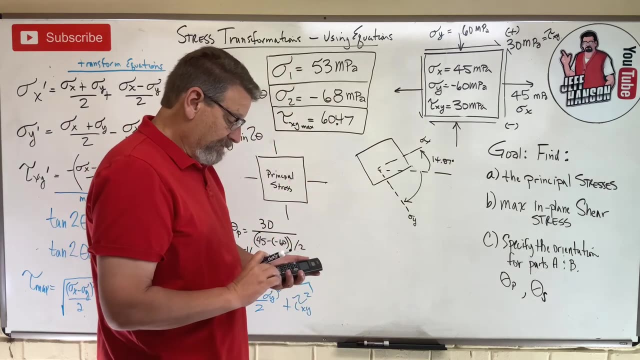 way, because both of those are going to be principal stresses, okay. So if this one is sigma x, then this one down here is sigma y, and those two are 90 degrees apart. so guess what this angle right here is? okay, It's going to be 90 minus 14.87, okay, Which is. 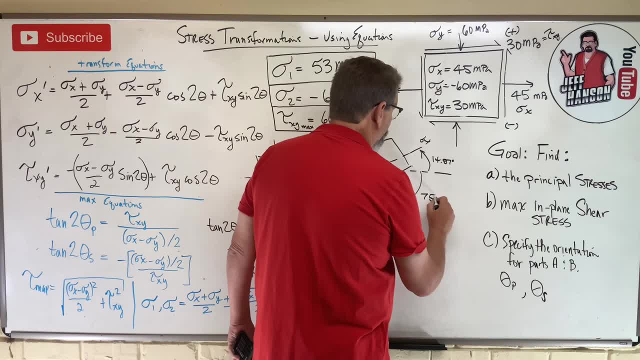 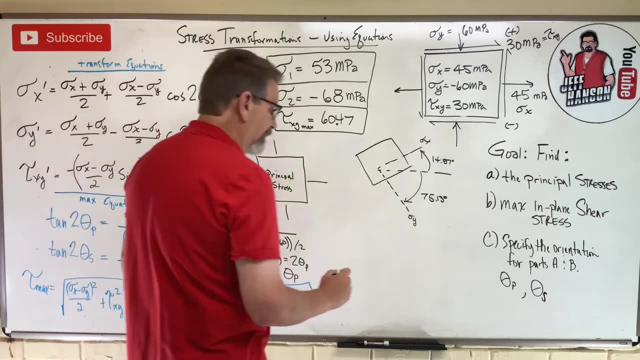 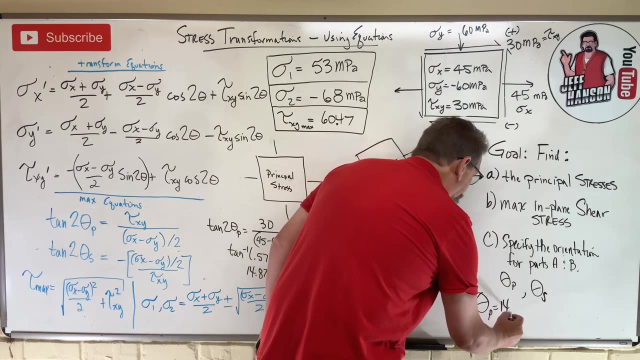 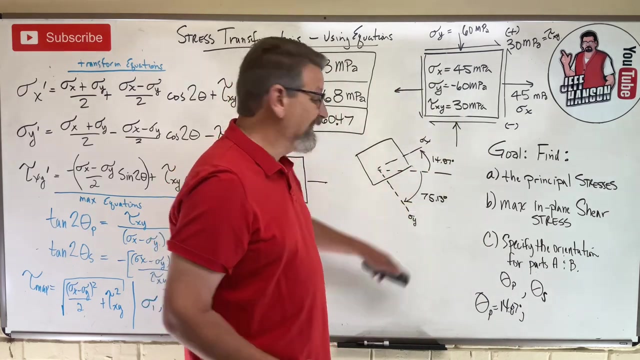 75.13 degrees. okay, And so sigma p, I would write it like this. I would write it like this: Theta p, theta p, theta p is equal to 14.87 degrees comma. and then the 75, which direction did I have to rotate to get there, Remember? 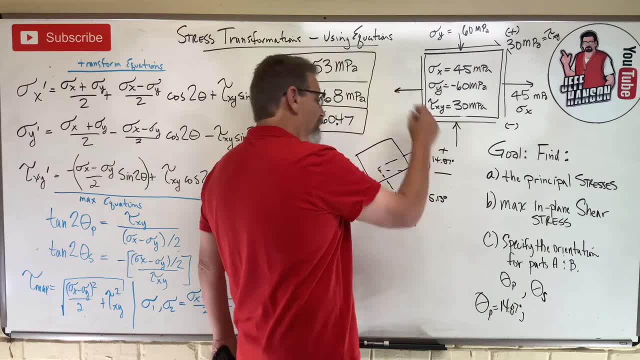 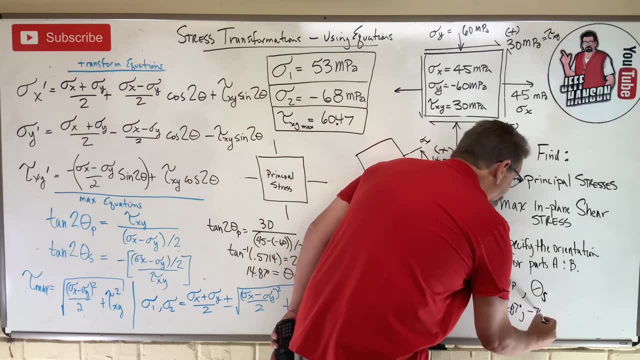 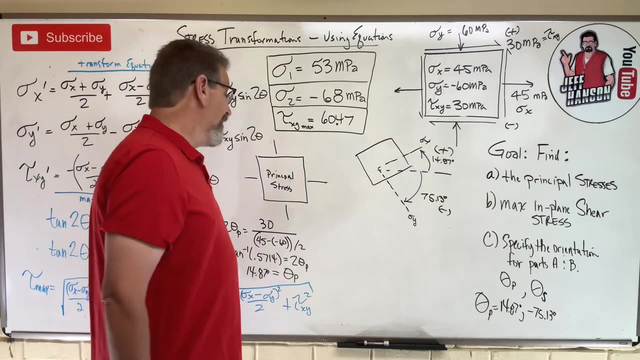 this is the positive direction of rotation: zero degrees, 90 degrees. This is the negative rotation direction, So I'm going to put negative 75.13 degrees. That's the proper way to write that. okay, So now I've got both those angles. Now let's go back On this stress element. 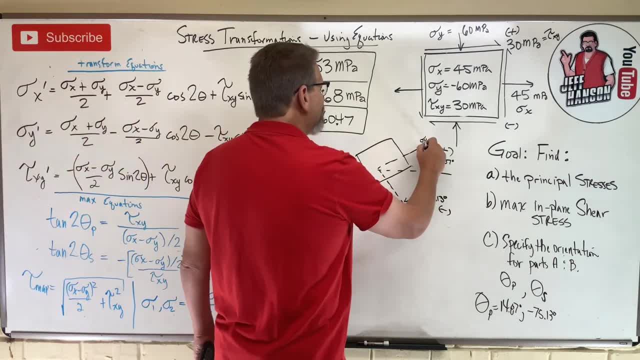 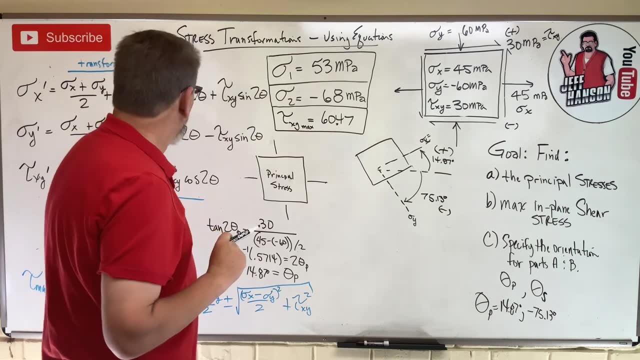 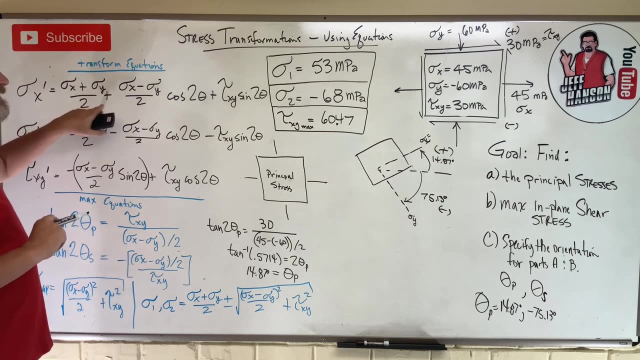 right, which is this new guy here? sigma x, is sigma x 53, or is sigma x negative 68?? Well, I don't know. Well, let's look at this equation up here. okay, If I take the numbers that I just got and plug into here and I put in the angle here, 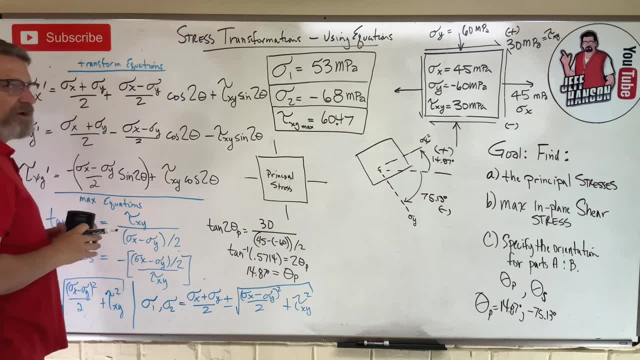 right, it will output me a number over here And if I take this top equation, you can try this on your own. okay, If I take this number up here and I put in for sigma x: 53,. no, I'm sorry, I put in sigma x. 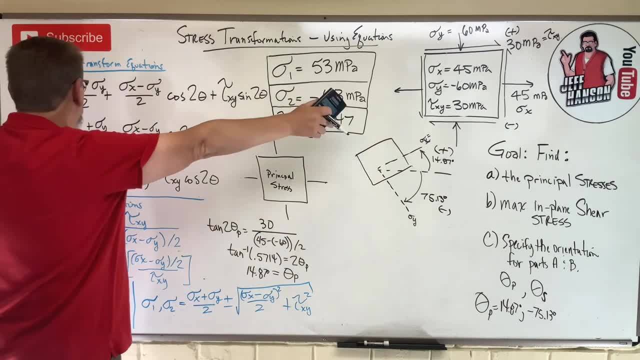 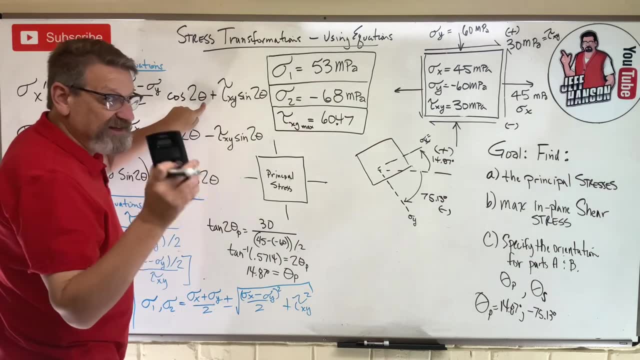 because this is not prime, this is untransformed right. I put in 45, I put in minus 60 there, 45 there minus 60 there. I put in 14.87 there and 14.87 there. what does sigma x prime give you? 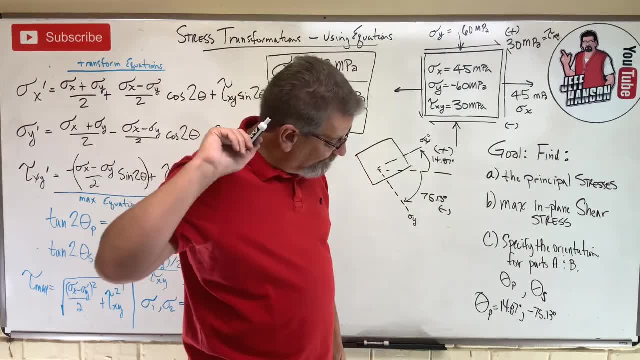 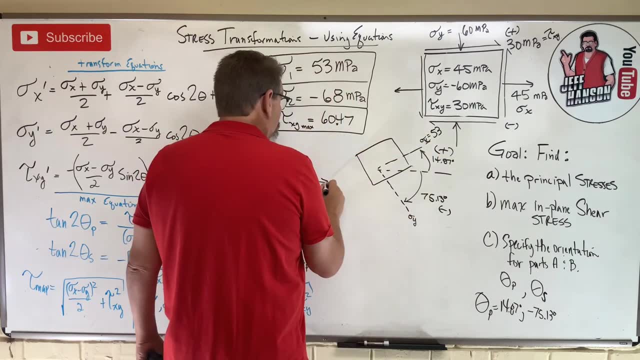 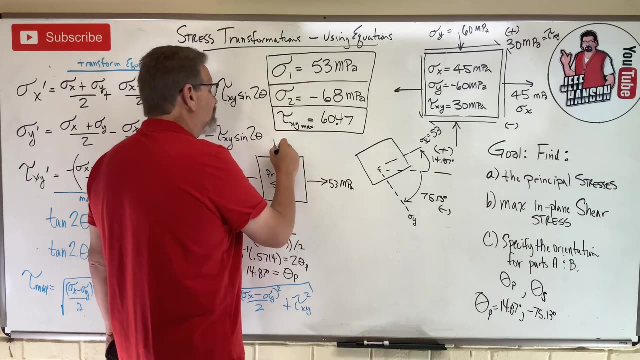 What does it output? I'll tell you what it outputs: 53, okay, So this guy here is 53, let's put it over here: 53 megapascals. and this guy up here in compression right, is negative. 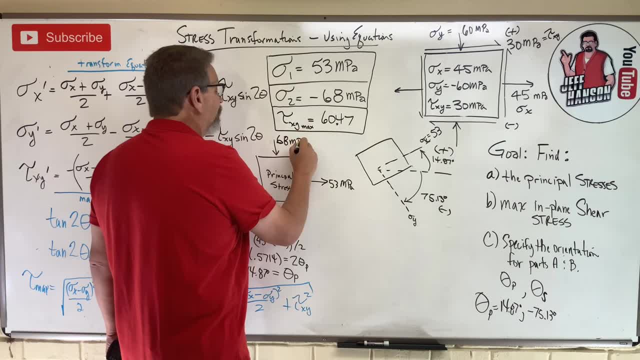 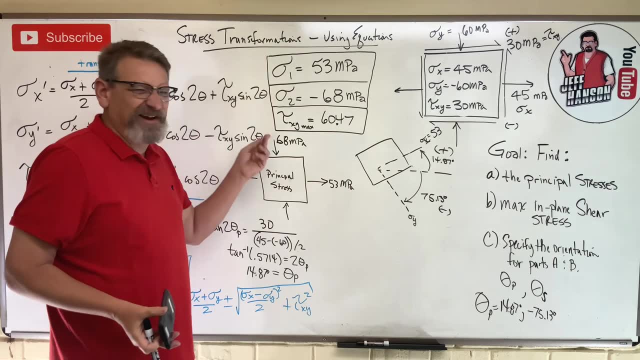 no, we don't have to put a negative, do we? 68 megapascals? Why didn't you put a negative? Because the arrow tells me it's in compression and I know that compression is negative. right, So if I put a negative there. 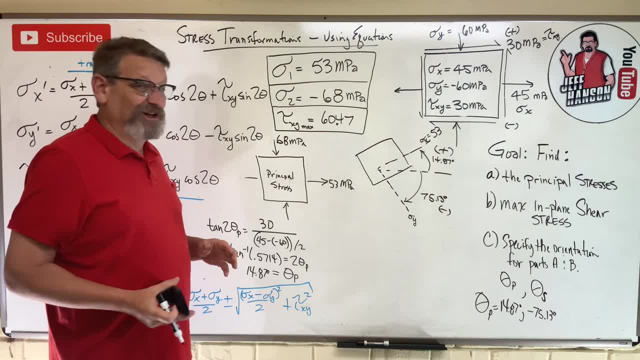 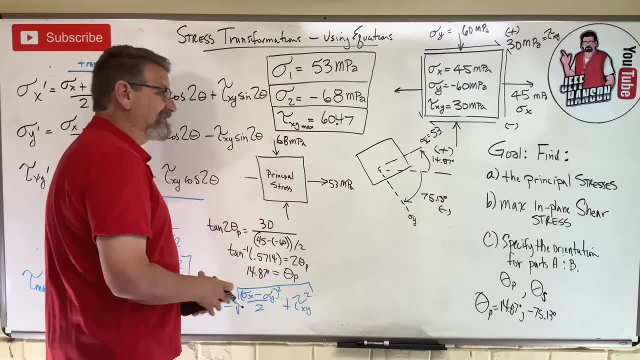 it's almost negative, right? So if I put a negative there, it's almost negative, right, Having a double negative, isn't it? This is a lot to follow, isn't it? y'all? Are you sticking with me? So that would be my stress element for the principal stresses. What would the shear stress? 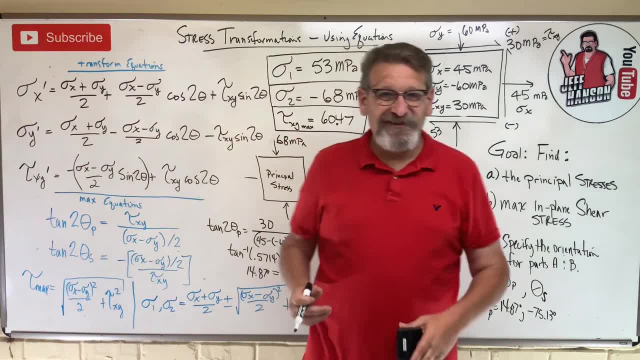 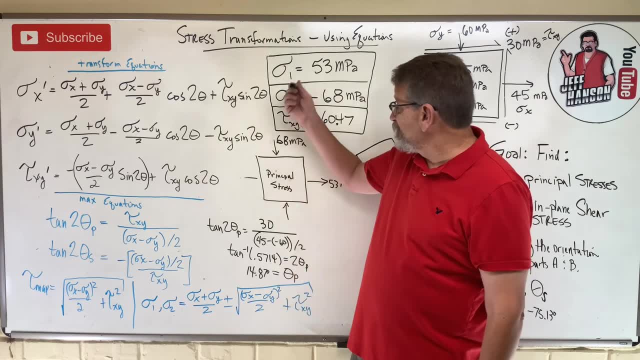 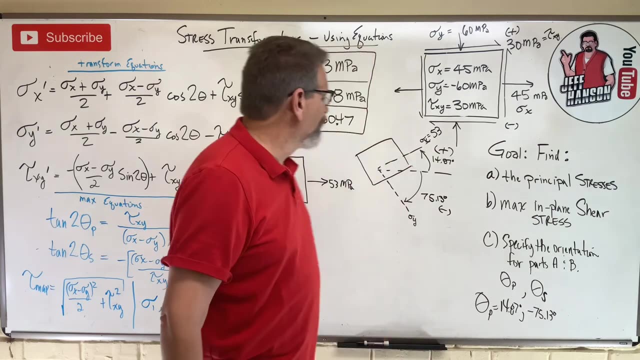 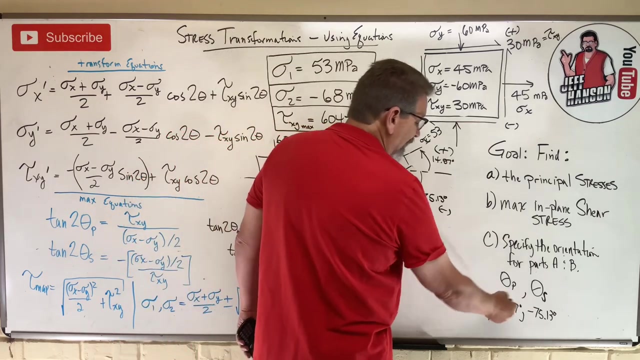 be on that Trick question, right? Did you fall for it? Trick question, Remember, when you're at the principal stress, which is these guys, which is those guys. tau is zero, It's zero, It's a trick, It's a trap. That's what Admiral Ackbar would say. okay, So notice this, These two angles, right. 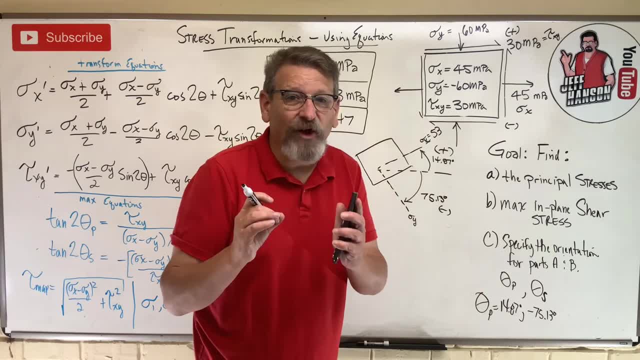 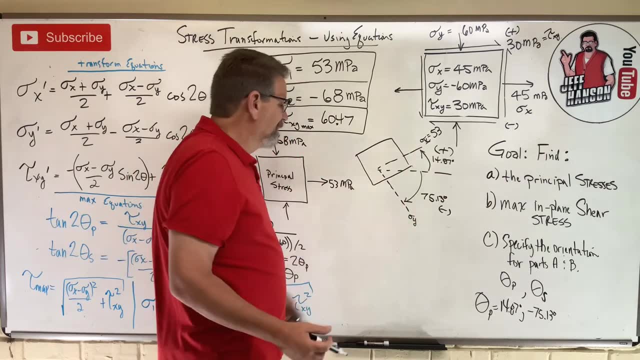 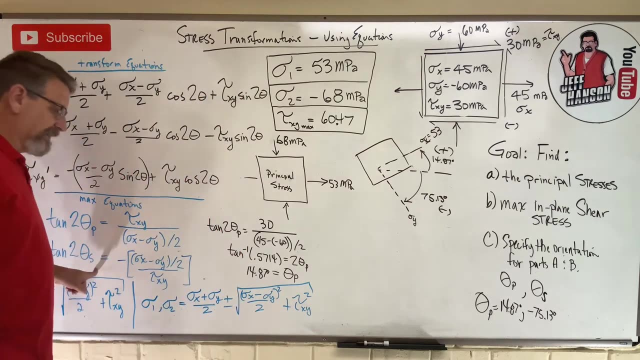 here for the principal stresses: always, always, always, add up to 90 degrees. okay, Because one's x and one's y, right, All right. So now that we found that, let's find one more thing, and let's find this guy. What is the angle where tau max occurs? 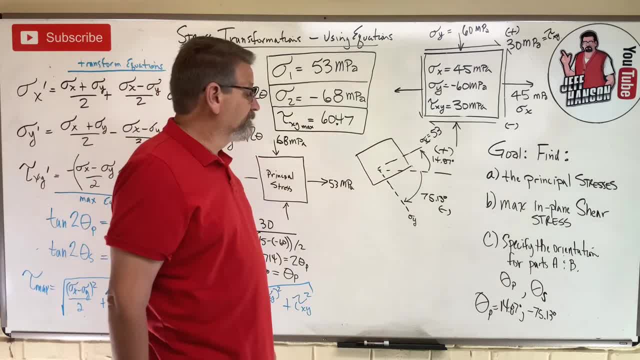 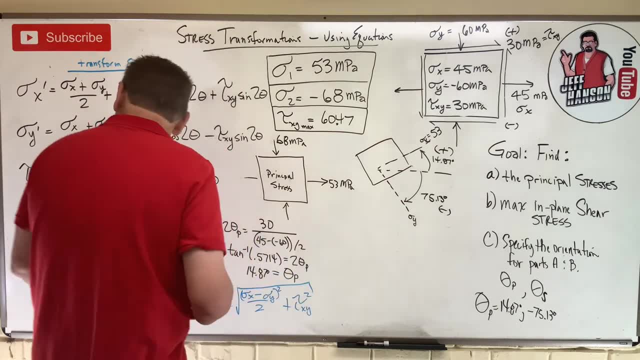 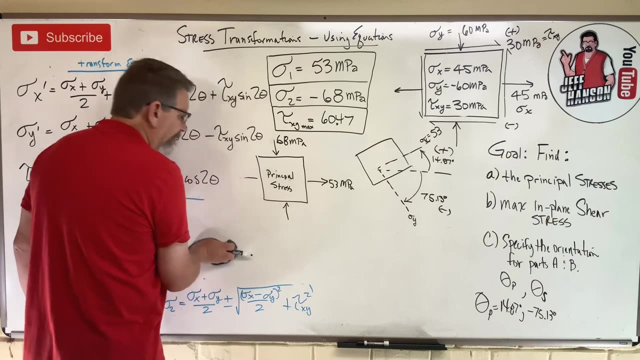 does not occur at 14.87.. Now, I already know, because I, because I know, I already know the angle, but let's see if we can calculate it. Okay, Let's erase something here. Okay, Let's erase all of this. Okay, And you know what We'll erase? uh, yeah, we'll erase this too. 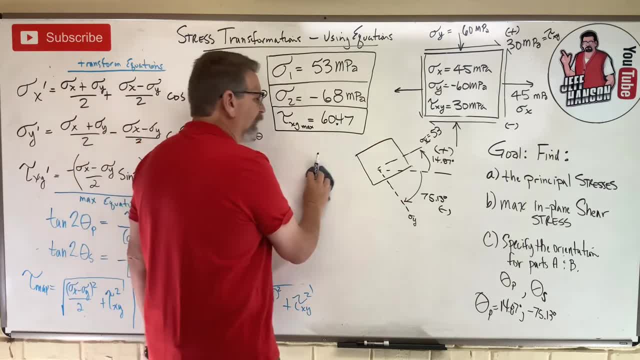 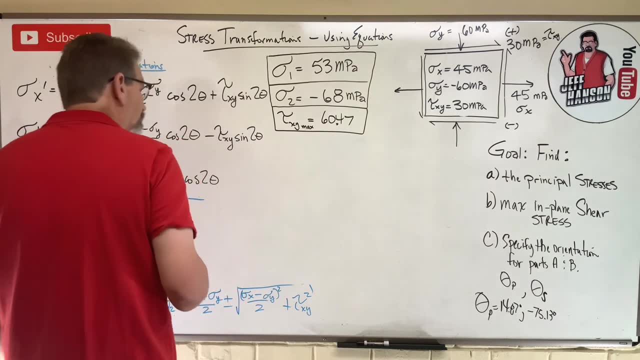 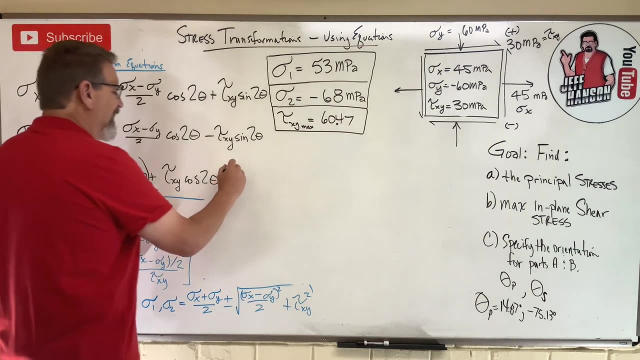 Okay, You have the luxury of just rewinding if you got lost, don't you? That's so nice, I know, right, Okay, So here we go, We're doing this guy down here. Okay, So tan two, theta S- this is not theta P- is equal to okay, here we go. The negative. 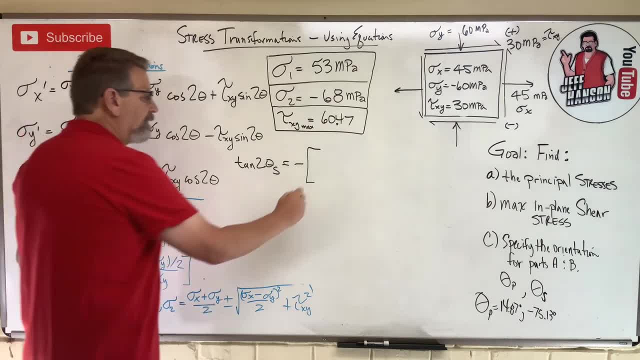 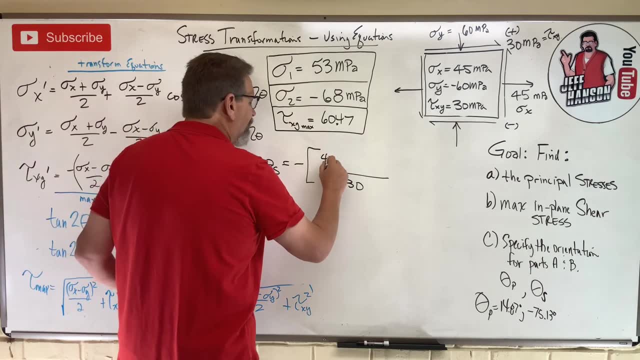 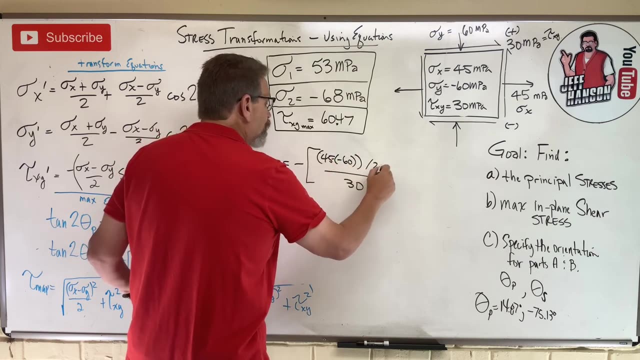 it's the negative reciprocal of this tan Top guy, isn't it? Who's on the bottom down here? 30.. Who's on the top? Sigma X minus sigma Y, So 45 minus a minus 60. And then all of that divided by two. Okay, All right. What is that? 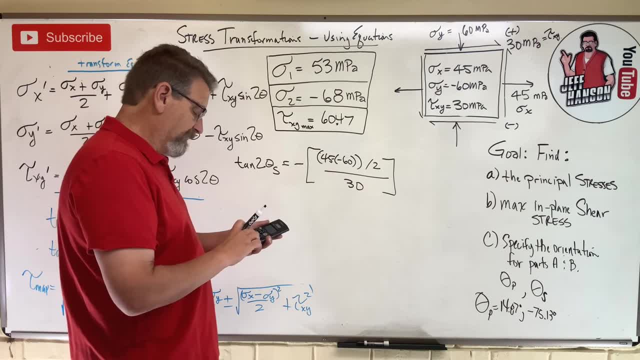 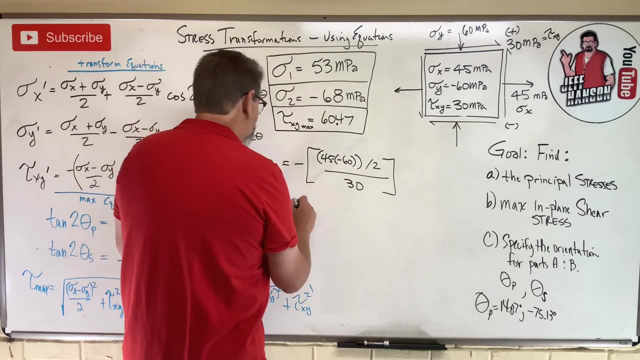 Minus. a minus is a plus. So again, that's 105 divided by two equals, not 3.16.. 105 divided by two equals 3.16.. 2.5 divided by 30 equals 1.75.. So that's negative 1.75.. So if we take the tan inverse of that, 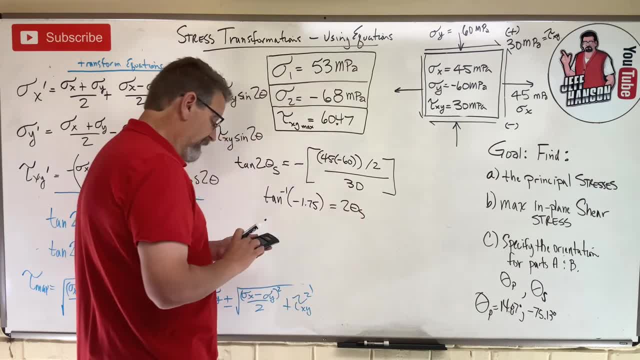 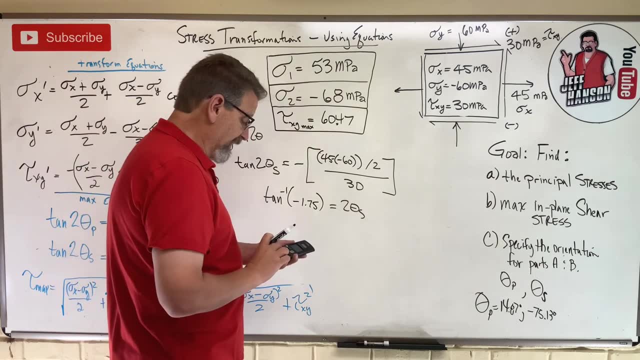 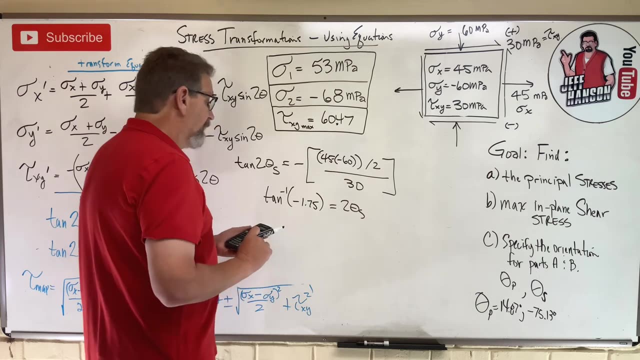 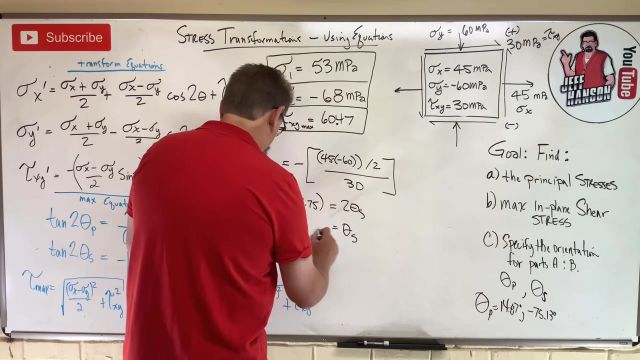 equals two theta S. So inverse tan of that- Oh oh, I did it wrong- Inverse tan of negative 1.75. there we go. And then, divided by two, right, Divided by two equals, So theta S is equal to. 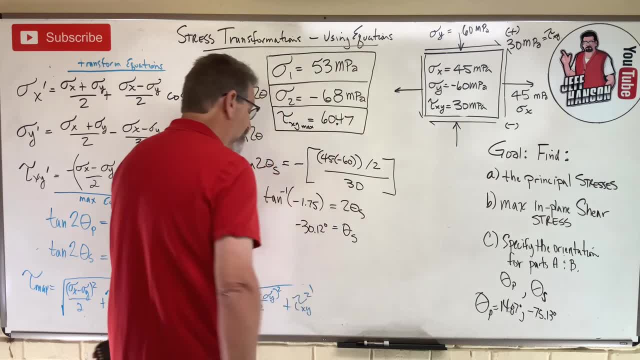 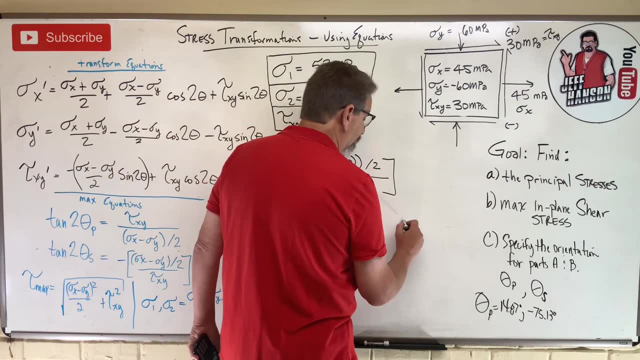 negative 30.12 degrees. There you go. So what does that say? You want to get to the maximum shear stress. you got to do this. Here's zero degrees, right, Here's the new one, the new angle. You got to go this way: 30.. 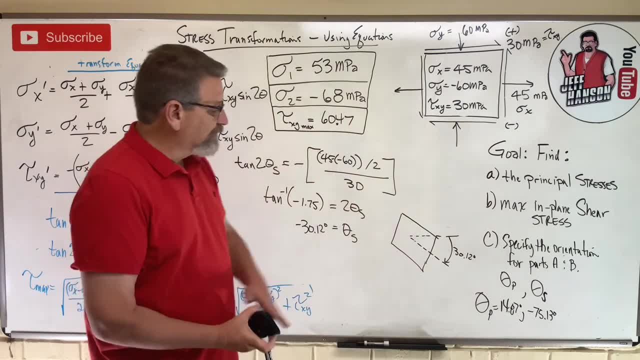 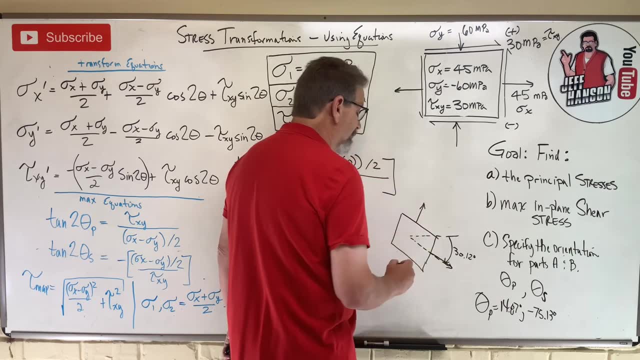 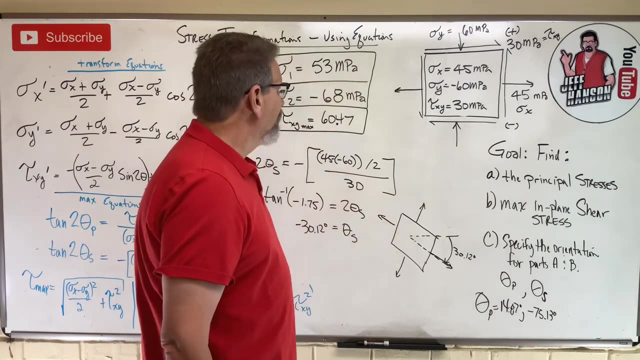 30.12 degrees right, Negative, which means you got to rotate clockwise. So now, this is my X face, right, This is my Y face. Now remember what we said. What are these two guys here? What are those two guys? Well, you add these two together: 45 plus negative. 60 is how much. 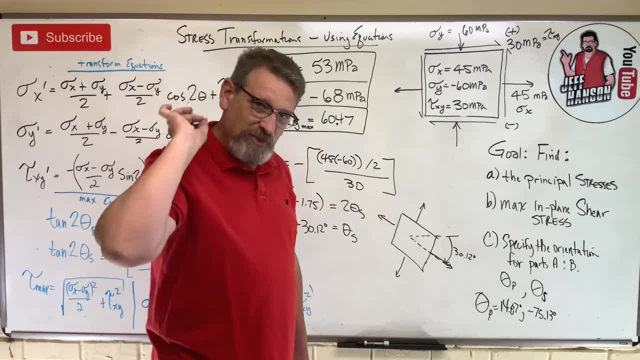 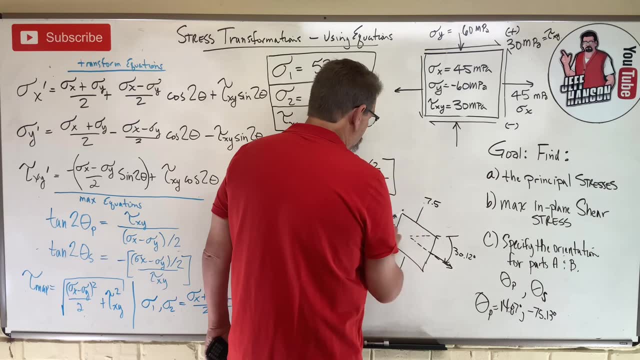 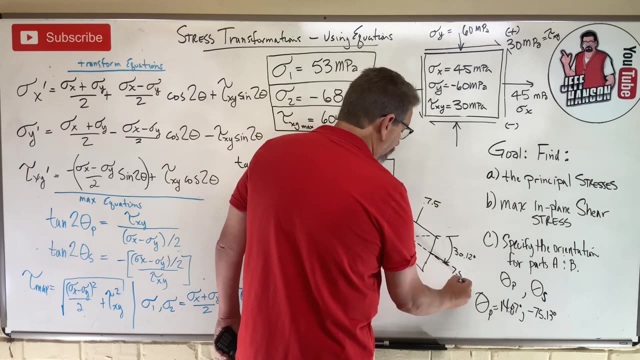 Negative 15.. Negative 15 divided by two is how much? 7.5 to the negative. What does negative mean? Well, I drew it wrong. is what it means. I drew it in tension, didn't I? But guess what? It's in compression. It's in compression. 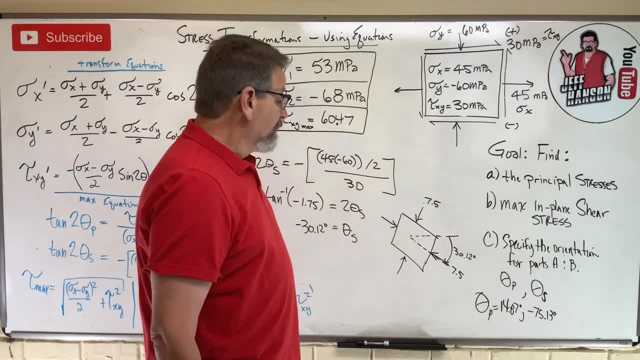 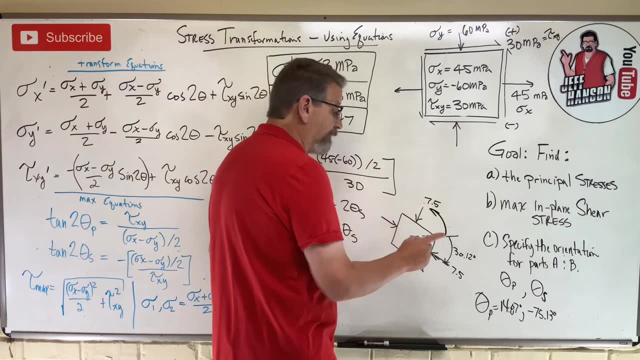 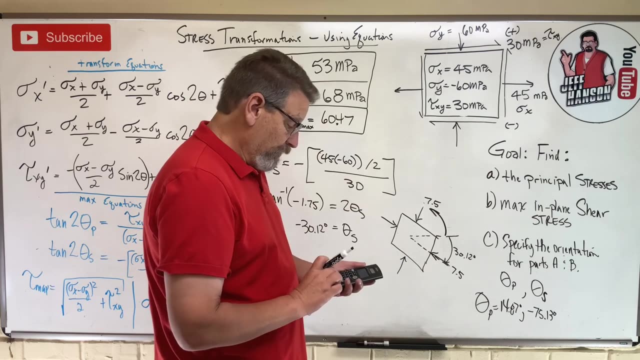 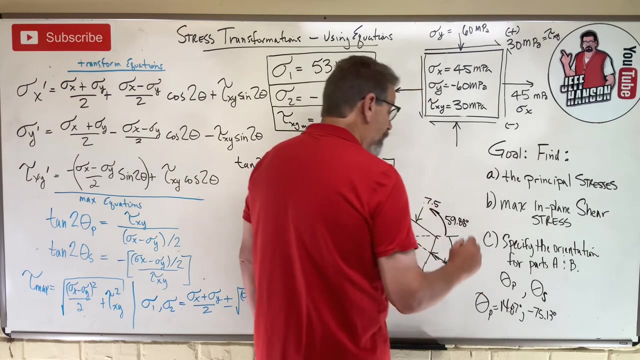 in compression in compression. okay, So same as we did down there. Guess what? This is up here? This is the other theta S angle: okay, And it's just what. It's 90 minus 30.12. answer which is: oh, 90 minus 30.12, 59.88, okay, So just like we did down here. 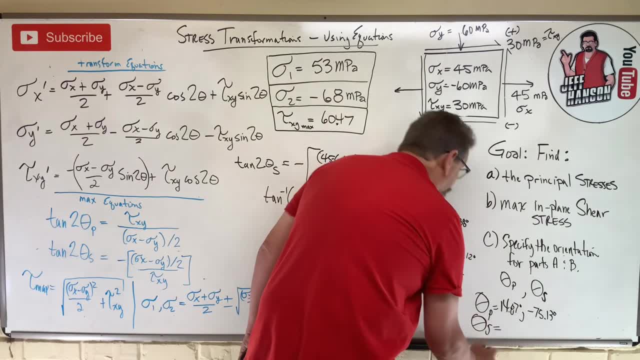 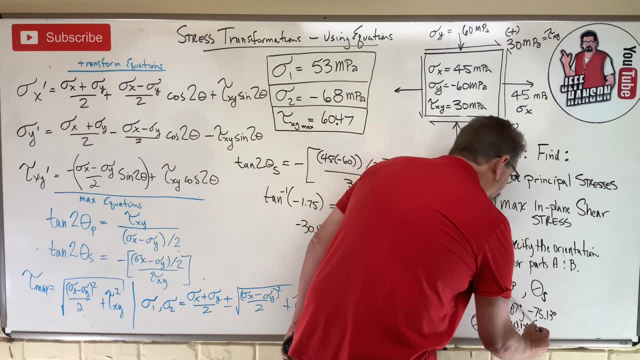 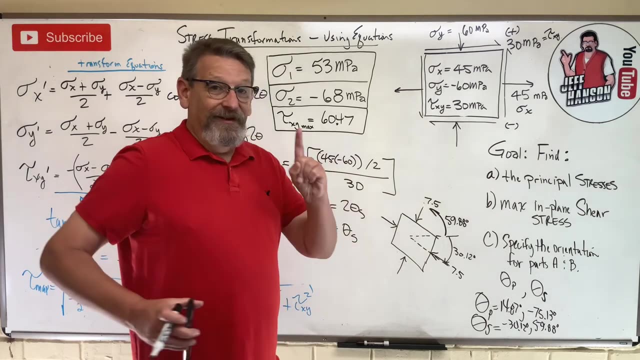 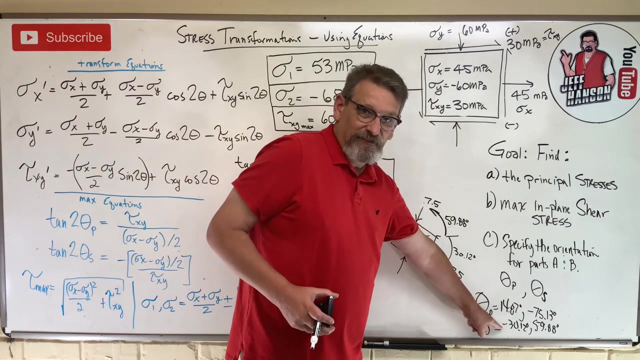 watch this. Theta S is equal to negative 30.12 degrees, comma 59.8.. 58 degrees. okay, I gave both of those angles. Now one more thing here. This is true always. okay, What is that plus that 45 degrees? Those two always add up to 45 degrees. 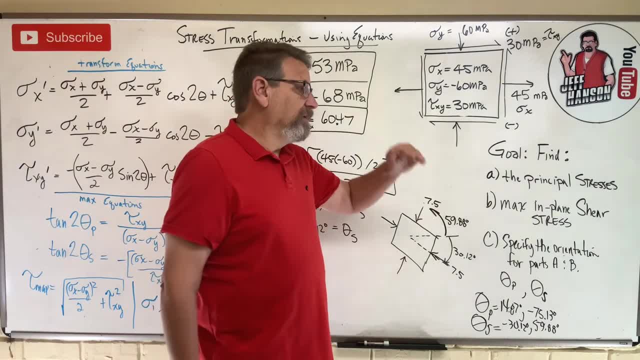 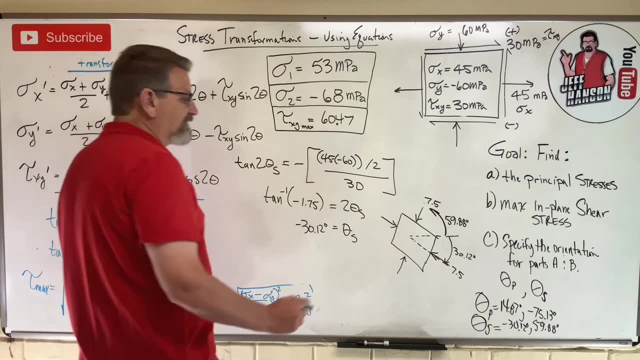 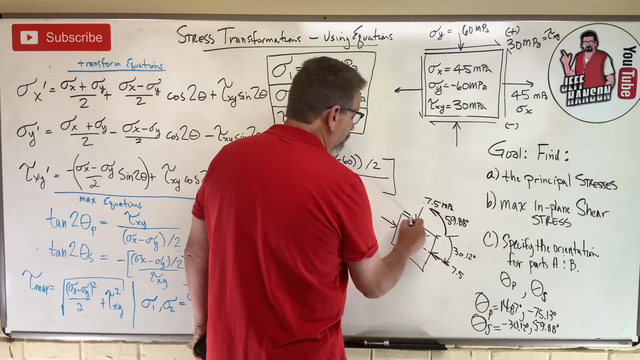 So the difference between the theta P angle and the theta S angle is always 45 degrees in real world degrees. okay, All right, And notice this, All right When I'm at the maximum shear stress, which is what Maximum shear stress?